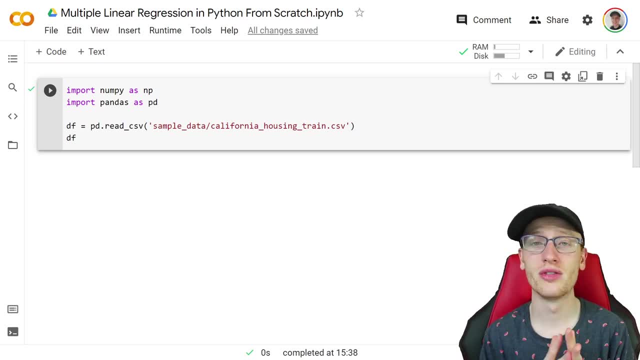 any of that stuff. This is intended as a beginner tutorial for machine learning and particularly in the idea of multiple linear regression. So I want to note that, again, this is from a machine learning point of view. there is lots of other topics in from a statistics point of view that you could talk about for multiple linear regression, but we're not going to really cover that. 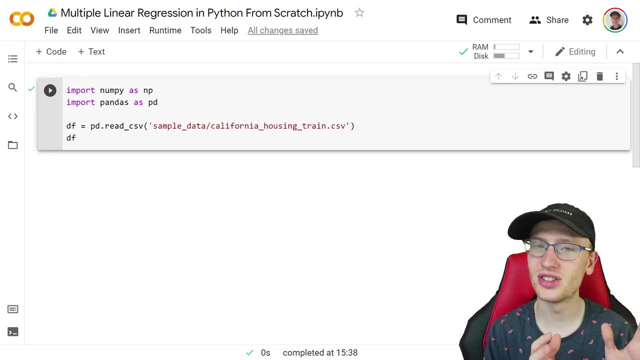 If you want to cover that stuff, then I would go to do a statistics undergraduate degree or at least read a statistics book on regression itself. okay, So let's get started. I actually got started a little bit prematurely. here We have import NumPy as in P, import Pandas as PD, and here is our data set. We're going to use the same one. we used 4-1,, 4-1, and 4-2.. So let's go ahead and get started. I actually got started a little bit prematurely. here We have import NumPy, as in P, import Pandas, as in PD, and here is our data set. We're going to use the same one. we used 4-1,, 4-1, and 4-2.. 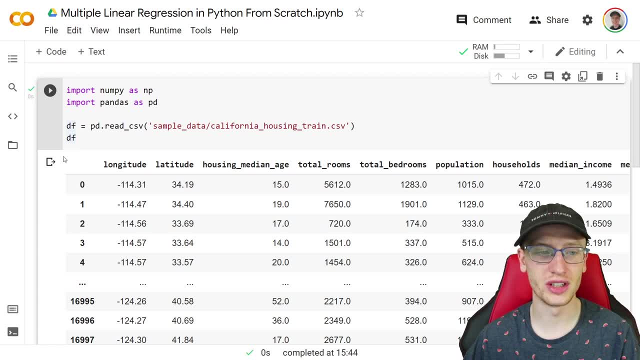 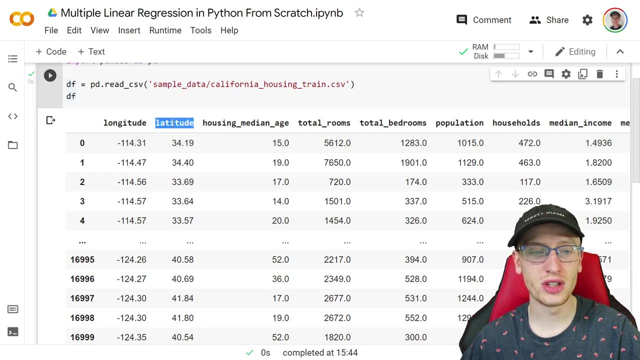 for the other one, which is the California housing training data set. So remember that each row is some location in California. It has a longitude and a latitude, a housing median age, total rooms, total bedrooms and so on. It has many of these variables. here I'm going to zoom out a little. 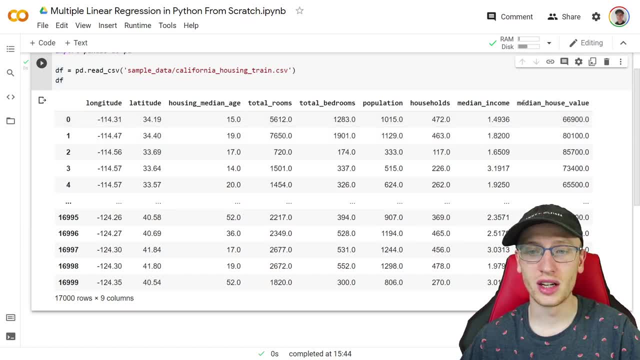 bit so I can scroll. I actually don't have to scroll now. So here there's the all the way up until the median house value. So last time we were predicting one of these variables- I can't remember, I believe it was either predicting total bedrooms or population. I believe we were. 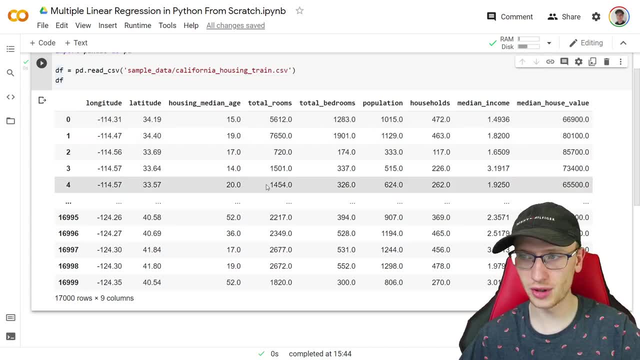 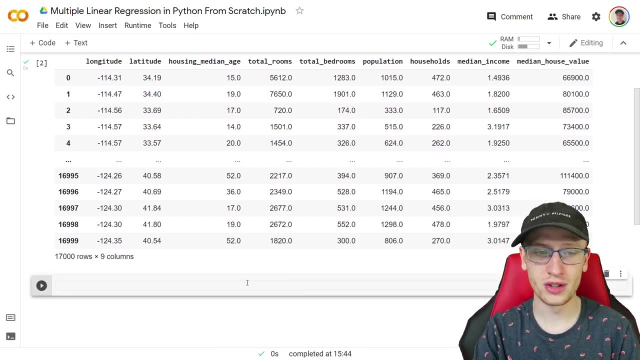 predicting the total bedrooms. That's what we're going to predict today, anyway. Okay, so we're first going to look at this idea called the correlation between variables. So if I do this thing and I have this stored in this variable called df- this data frame, panda's data frame- and if I do dfcore, 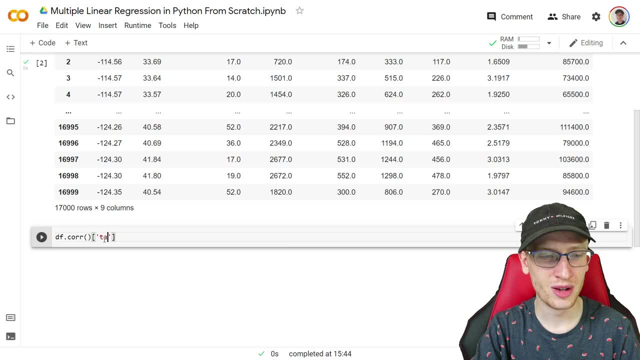 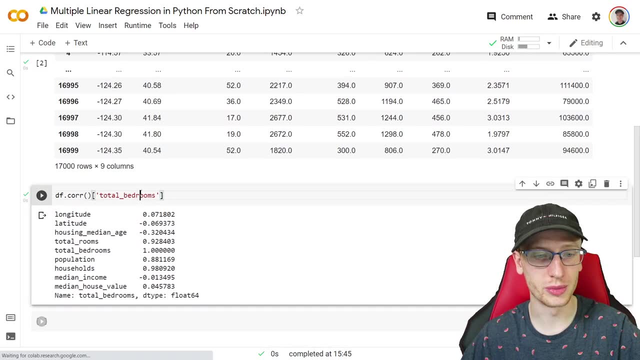 and I always think of my friend Corey because of core, but here. So total bedrooms, we're going to be trying to predict this variable. So we're going to be trying to predict this variable. So if I look at the core sub this variable, then what we get here is a series of values with 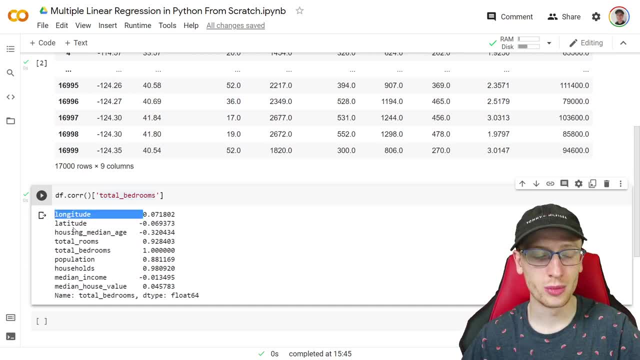 corresponding labels here, where we have the correlation between- and I'll explain that in a moment- between total bedrooms and longitude, with total bedrooms and latitude, all the way up until total bedrooms sub median house value. It also gives this correlation with itself, which basically: 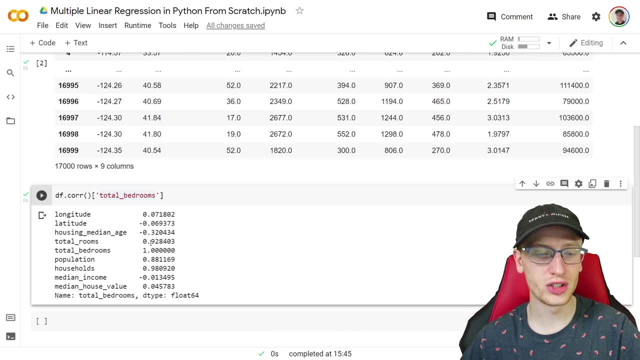 means it matches up perfectly. So these are all individual things where it's the pairing of total bedrooms and each of these variables. So if we look at it, for example, total bedrooms and total rooms, this means this value of 0.92.. Well, first of all, it's positive. 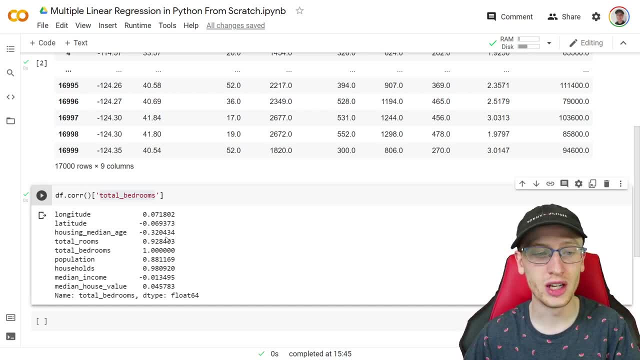 Okay, there's other negative values here, So this value could have been negative. It was positive. That means, as one of these variables increases total rooms, then total bedrooms would tend to increase as well. So we'd have like a positive, a positive slope and the negative ones, So that 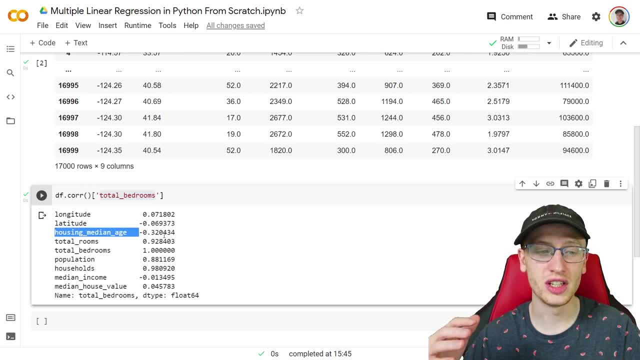 means we have a negative slope, As housing median age tends to increase. we see that the total bedrooms seems to decrease And that actually makes sense If we increase the age or how, basically the, the oldness, oldness- I don't know if that's a real word- how long these houses have. 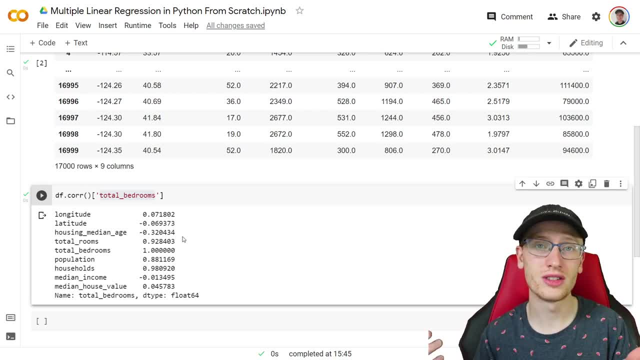 been around. we tend to have less bedrooms, And that makes sense, because you know we probably are making rooms with more bedrooms now than we did used to be Okay. So there's lots of these correlations of 0.0.2 and 0.0.3.. What's that mean? Well, 0.1 or 0.1 and 0.3 are less than 0.2,. 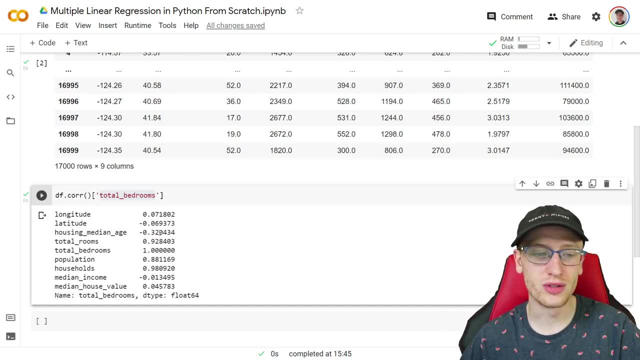 or they're closer than 0.3 or 0.4, or 0.3 to 0.5, or 0.5 or 0.5.. So that's a lower correlation. So 0.7 is a lower correlation than 0.2.. So that means 0.9 is closer to 1. And 0.7 is closer to 1.. 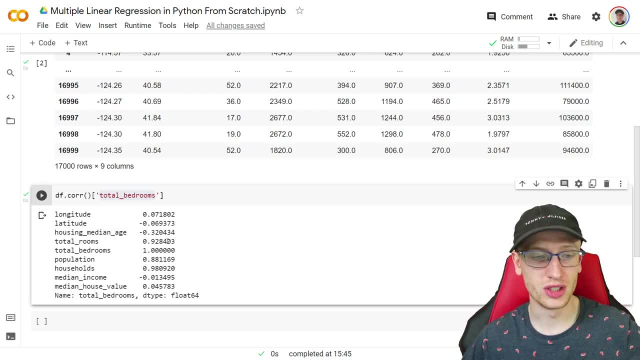 So 0.7 is not close to 1.1.. So if I limit this 0.1, 0.8 to 0.2, and 0.6 to 0.5, I can limit it to that one. So there's lots of different correlations. These are either a positive correlation or a. 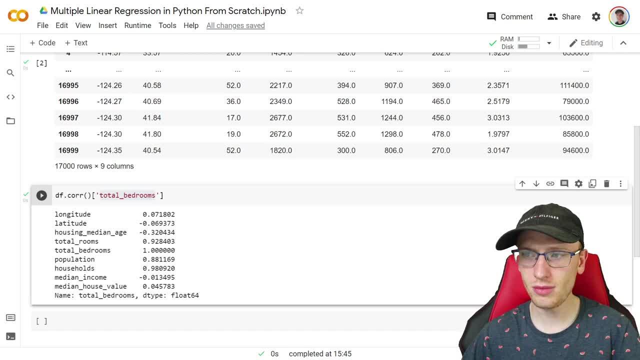 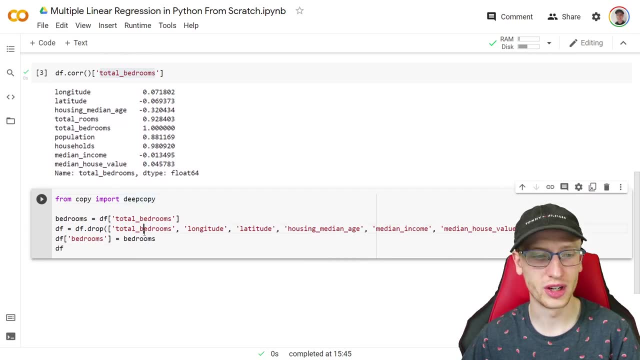 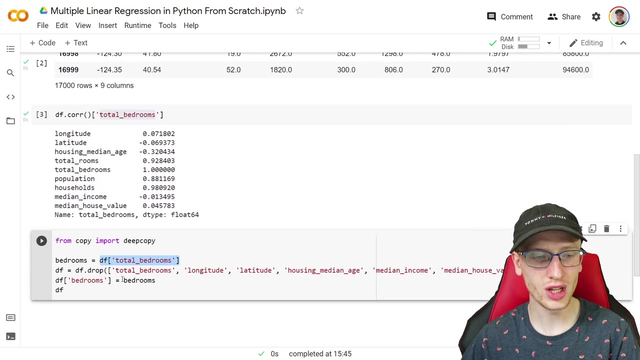 negative correlation, something here. but what we're going to look at today is- i'm going to just copy in this code for you: we're going to look at. so first ignore, don't worry about this too much right now. if we set bedrooms equal to this variable here, which is just the total bedrooms column, and then we drop, 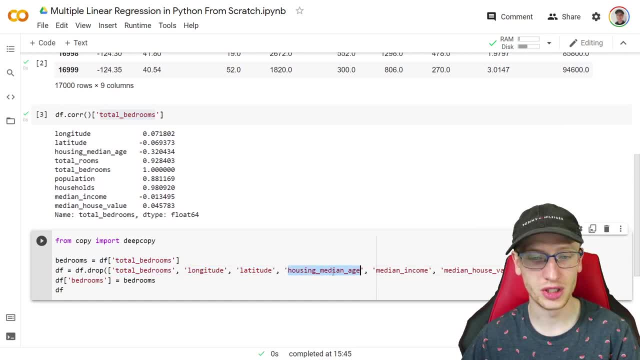 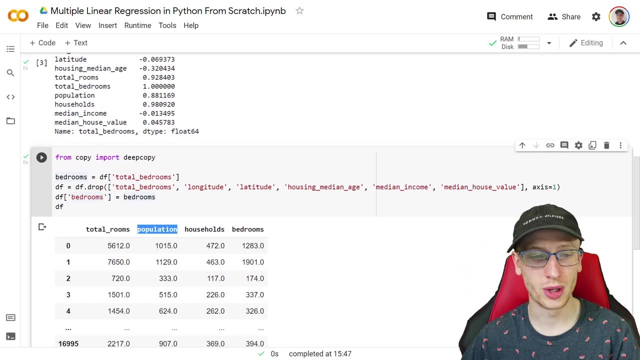 total bedrooms, longitude, latitude housing, median age, median income, median house value. why did we drop these columns so that it turned into this, where we have just total rooms, population, households and bedrooms left over at the end? by the way, i placed that at the end on purpose, and that's how. 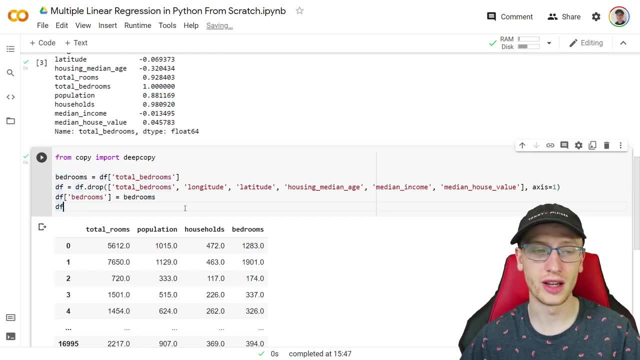 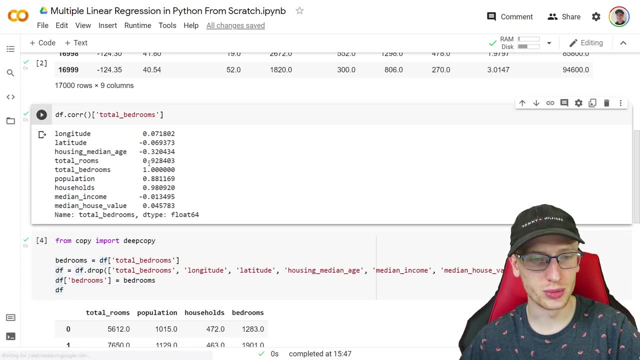 i did that did this is basically i dropped it and then i added it back in at the end, and so why did we do this? well, basically i only grabbed the ones that have a strong correlation. here i have total rooms: 0.92. i have longitude. i got rid of longitude and latitude because they were these small, very 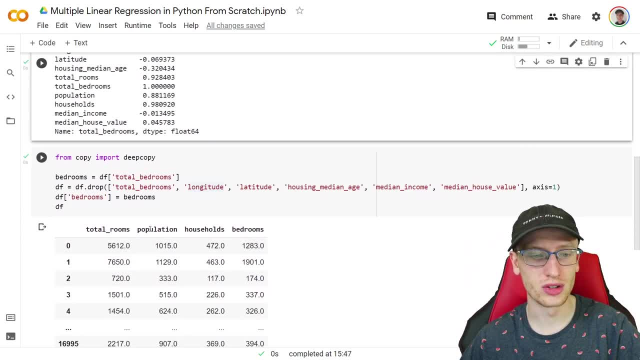 close to zero values. and yeah, we only kept the ones with the strong correlation: total rooms has 0.92, population has 0.88, household has 0.98 and i got rid of the other ones. okay, so i just did that with, uh, basically keeping that in a variable, and then actually i never even used this copy thing, so i 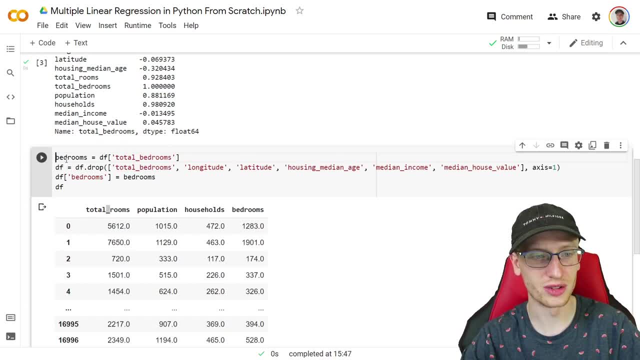 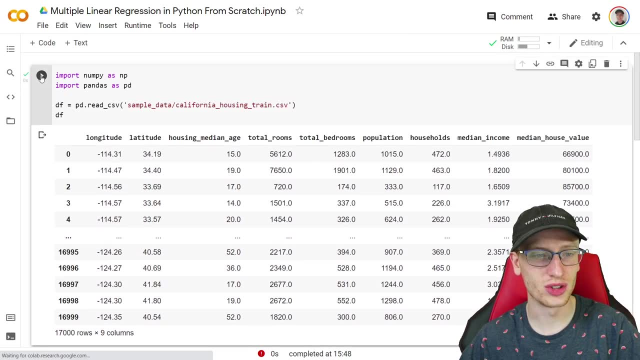 don't really know why i even kept that around, right? i don't. i don't think i ever used that. okay, so that says df the above exception, right? so this will happen if you start to run things by overwriting the variable name, and i'm just rerunning from the beginning to get that again. 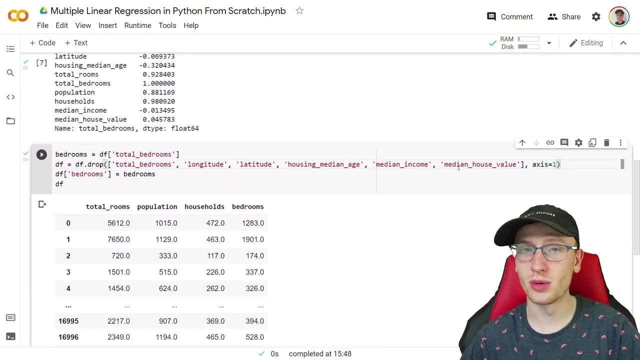 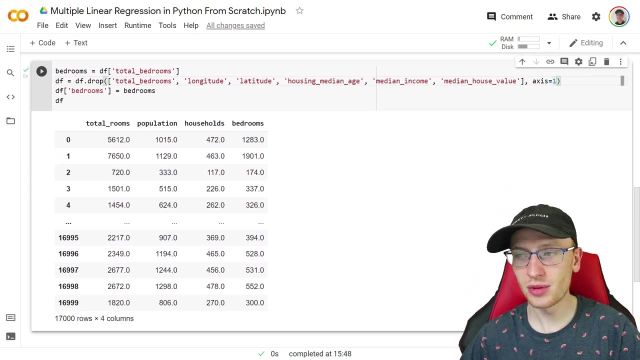 so we can do that and remember the axis equals one. this i threw in there because then it's- uh, it knows for sure to drop the columns in particular. so, anyways, we got the data set down to this and we want to perform a multiple linear regression. well, we're not quite there yet, and again. first, 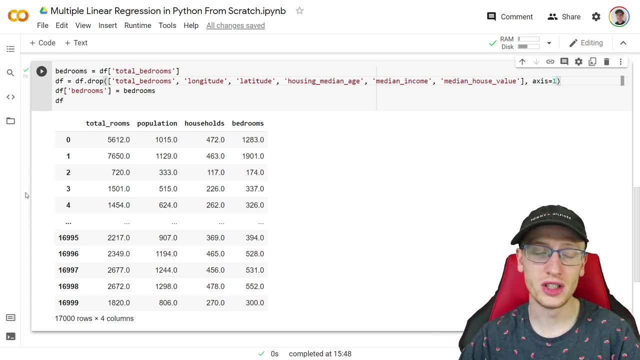 like we did last time with simple linear regression. we do want to see how we'd- uh, how we would use scikit-learns like proper library, which is how you'd actually go to do this if you were doing it in practice- and we'll get to that shortly, but for now i'm going to go ahead and do that and i'm 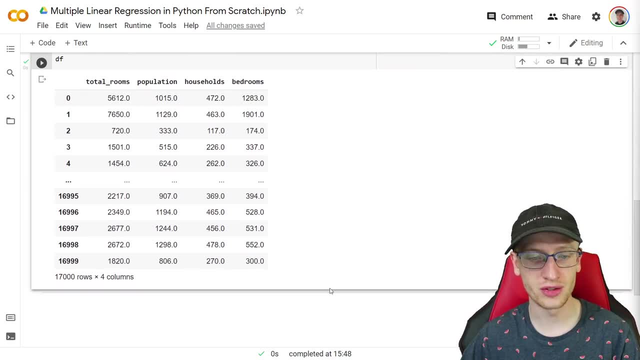 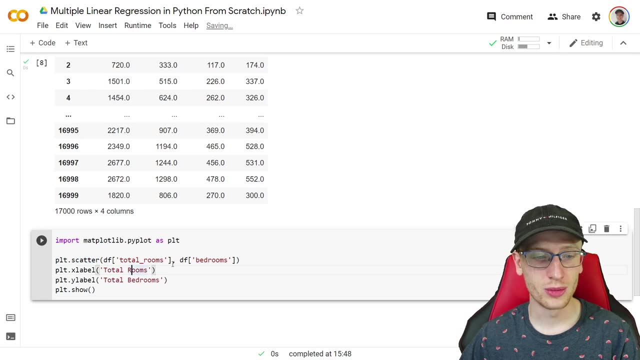 going to make some individual graphs and again i'm just going to copy some code in for you and explain that if we import map all lived up high plot as plt, that's our graphing library- and we do a scatter plot between the total rooms column and the bedrooms column. we can see here that yes. 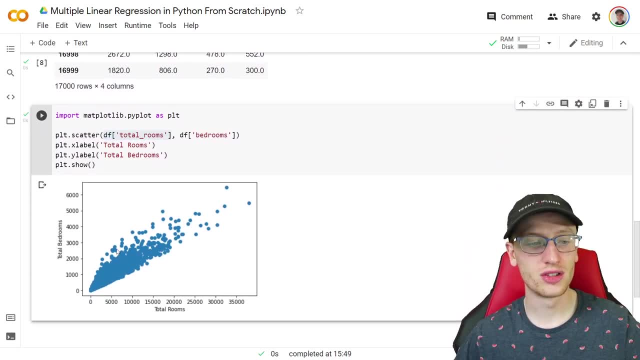 as we saw from the correlation, as total rooms tends to increase, the total bedrooms tends to increase as well. and now i'm just going to copy basically the same code. by the way, last time we didn't really use pltshow- you don't really need to in a jupyter notebook, but it 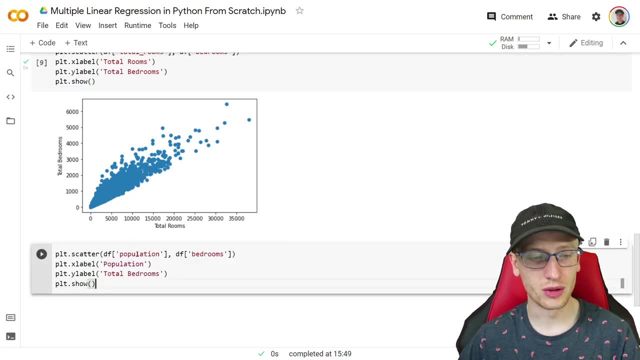 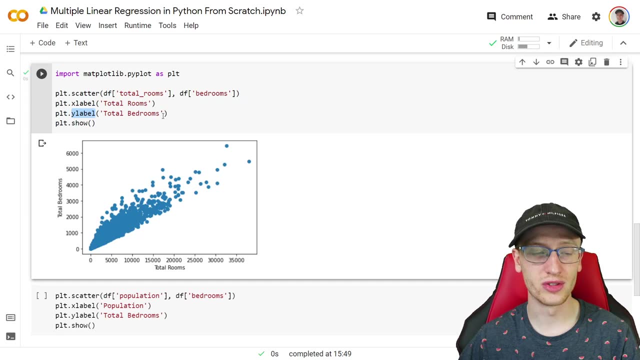 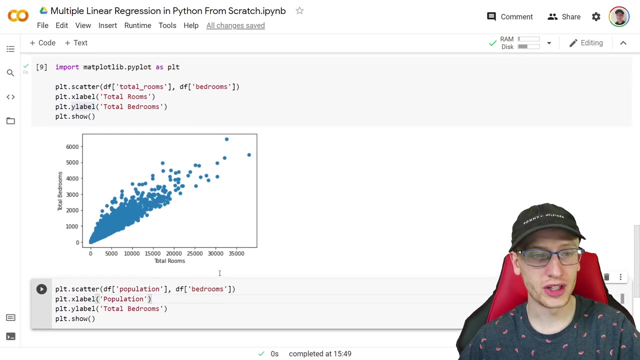 makes it look ever so slightly better. if i copy this in now: population in bedrooms, this is exactly the same thing, except i'm labeling, and you use x label for the x label, y label for the y, y, y label. i can't say that. um, then that labels them as well, and so now i'll show population in bedrooms. so 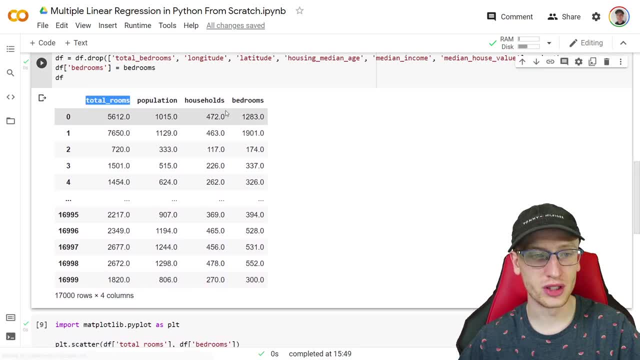 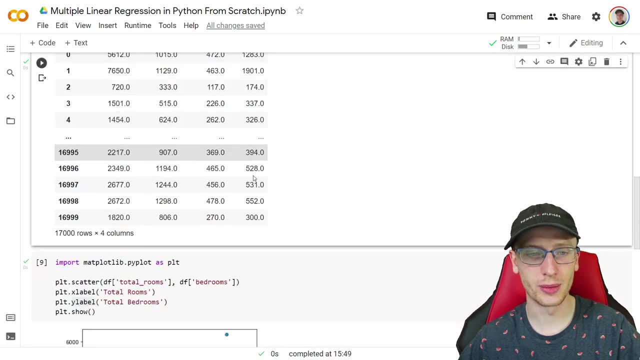 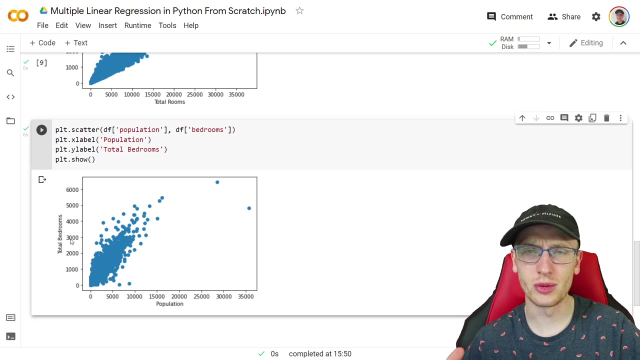 basically all i'm doing is plotting the individual graphs between this column and this column, this column in this column, this column in this column, because we're looking at how individually our inputs map to the outputs. so here i'll show it with, uh, with population versus the total bedrooms, actually generally. 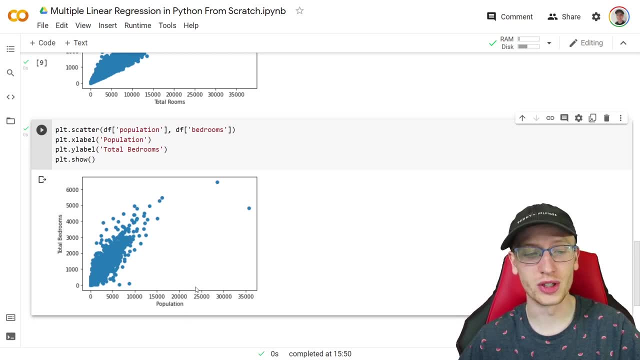 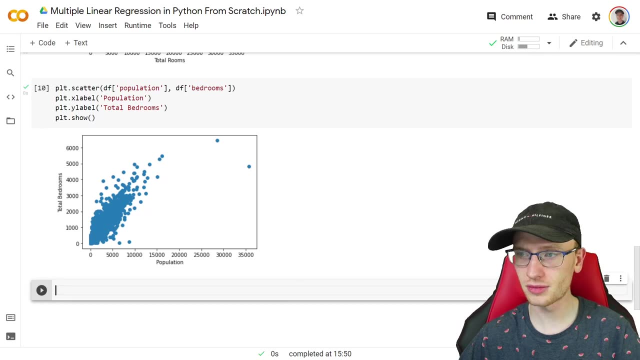 when you say versus, you usually say y versus x. you would say total bedrooms versus population. but not a big deal, we can see here. as population has increased, total bedrooms tends to increase as well. and then, finally, i'm just going to do one more, which is plotting households and bedrooms. 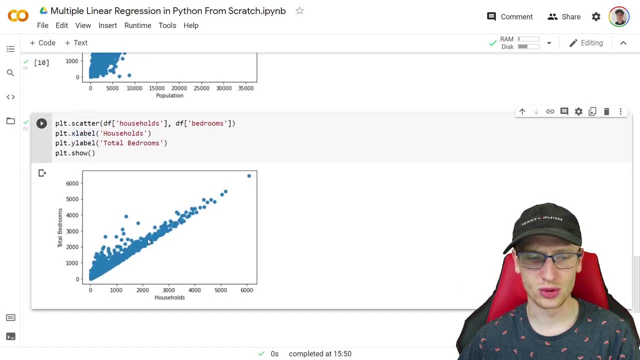 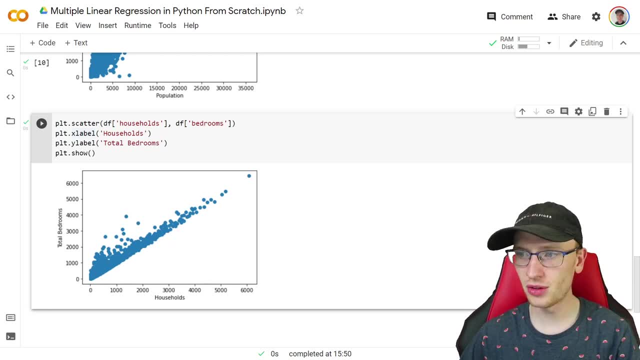 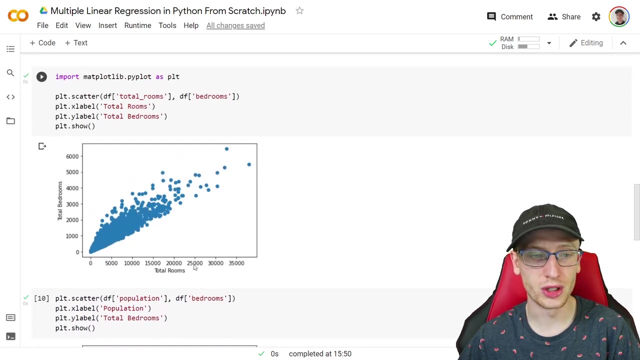 bedrooms increasing as well. okay, so why did i do that? not any reason in particular. it's kind of just to show some visualization for you now. uh, to show how scikit learn how- we'd actually make this multiple linear regression where we combine the results of household population, total bedrooms. 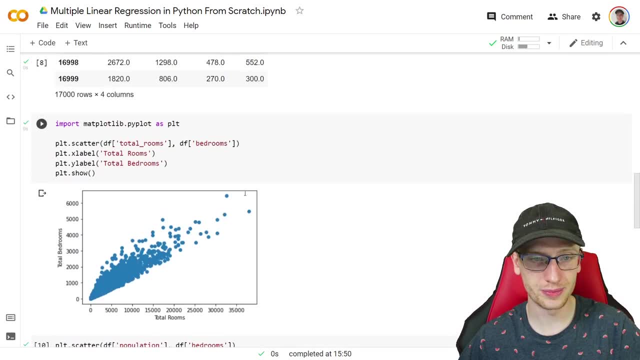 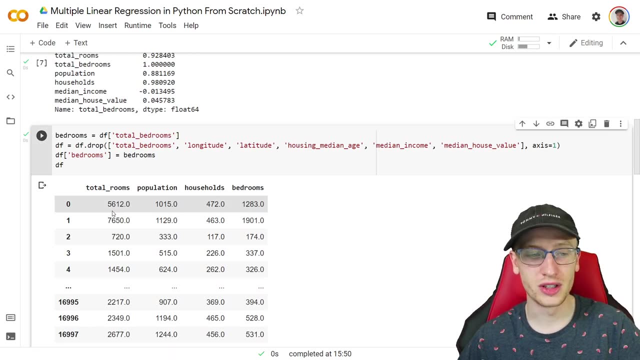 to try and predict the associated total bedrooms. value this column here. so basically you would do. what we're assuming here is that the relationship is: alpha plus some slope times, this value plus some slope times, this value plus some soap times. this value is roughly equal to this. so it's a linear relationship. we'll talk about that. if you didn't understand that, don't. 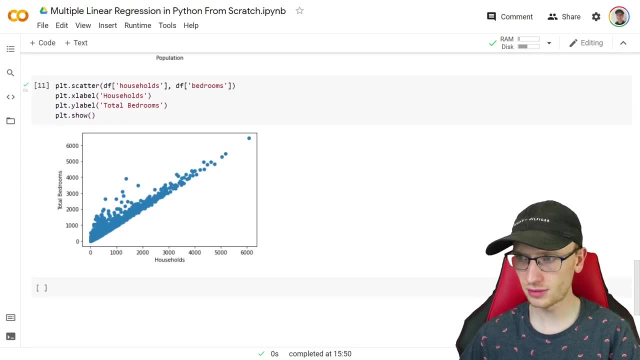 worry, we will absolutely revisit that idea. okay, but we're making a linear model and to do this, I'll actually start writing some code. df underscore numpy is equal to df. dot to numpy. why am I doing this? because we are converting to a numpy array and df numpy- numpy arrays have a shape, so we have 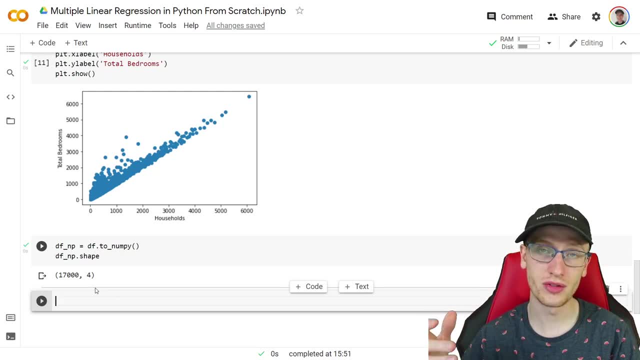 four rows and four columns, where that last column is our output or Y variable. the first three are different input variables. if I get x train and I'm writing train, because that's this is the data, so that's going to be used to train the model x train and Y train is equal to df numpy. I can do a little. 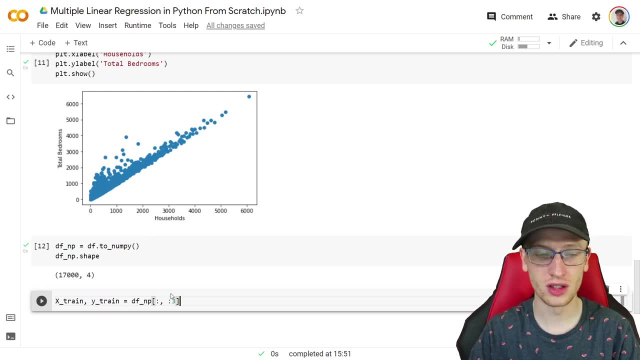 trick here: all of the rows and then up until the um. so remember, this is not inclusive, so basically it would grab. this means all the rows and this means: which columns do you want? i want zero, one and two, the first three columns. that's what that means. 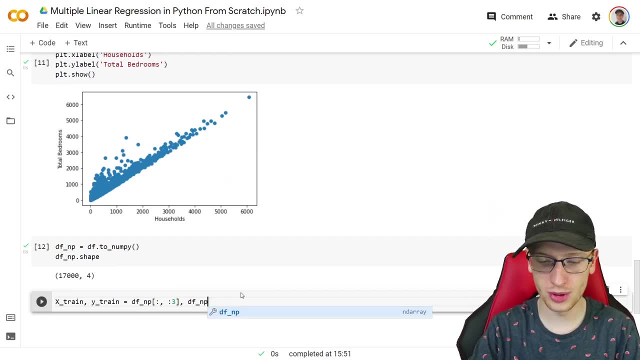 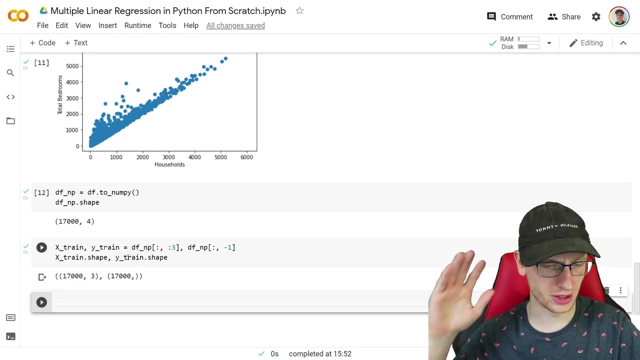 and we also have df numpy sub colon until negative one. okay, x train dot shape and y train dot shape, we should see that we have a 17 000 by 3.. i'm going to start calling this a matrix, because a matrix is really just a term for a table, but table without column names. in particular it's: 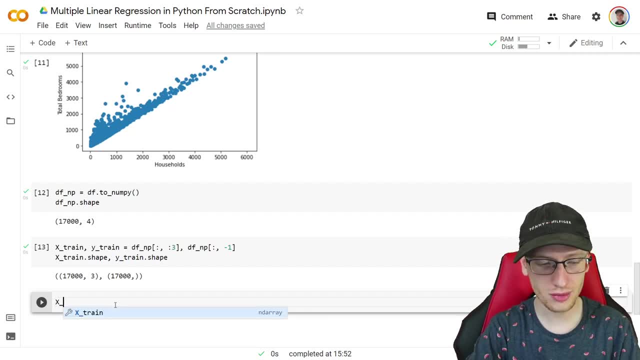 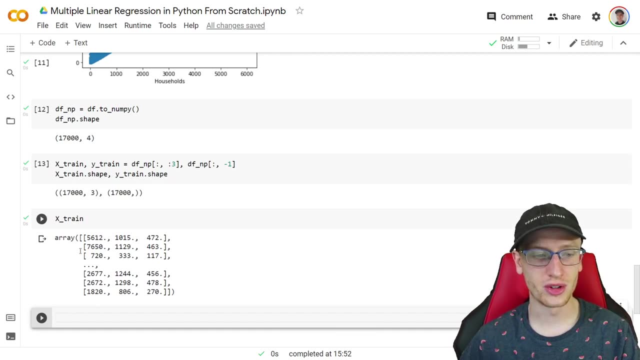 just values. so that's what we have here and you can see it. i can output x train. it's not going to open the whole thing is. it's very large, but we can see it has 17 000 rows going down and then three columns wide, so it's the same thing as our data frame, at least the same. basically this, this: 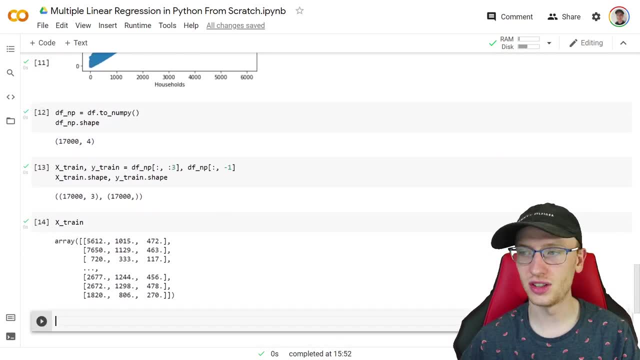 chunk this chunk here, but it's a numpy so that we can feed it into scikit-learn. now, if you remember well, we had this data frame and we had this data frame and we had this data frame and we had this from paper discovered. okay, and i'll just clean up this beautiful blank. but again, what we want, what 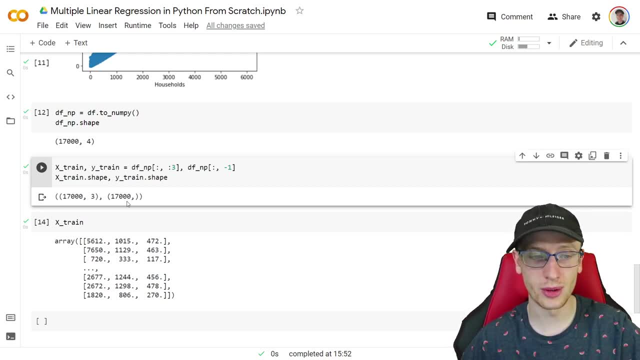 we want to do for scikit-learn last time was actually reshape it to be 17 000 by one, because this time, or last time, it was just 17 000 comma. the input was that. uh, the output is still that and that makes sense and we're happy with that. this time it's already in this form of there's. 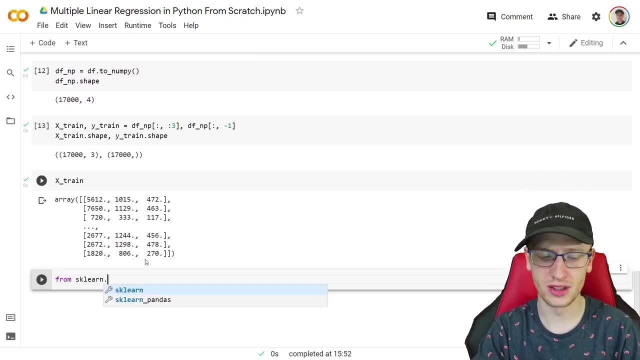 like another dimension here, 17 000 by three, because it is naturally a matrix, and this is why scikit-learn prefers that idea again. if that didn't make sense, i wouldn't really worry about regression And remember, what I'm doing now is not what we would actually do to implement it. 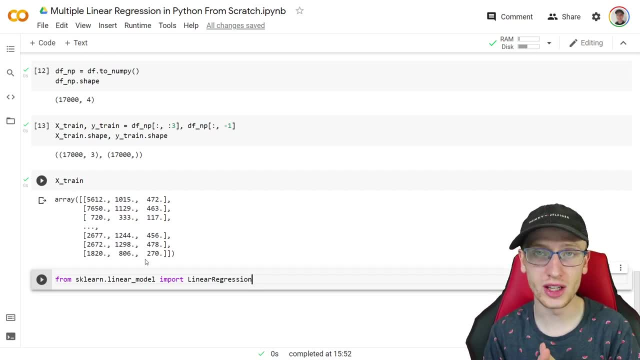 from scratch. This is just showing the idea of what we would do in when we're actually going to do it in real life, like after this lesson. if you want to go do it and make a linear model, this is what you would do, And so we're doing this so that we see how to implement stuff. 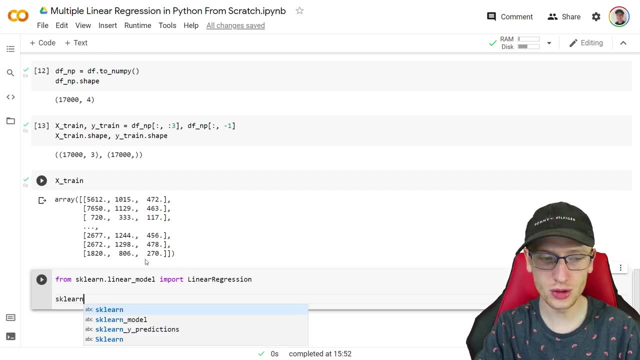 from scratch what we want to implement from scratch. So we'll make sklearing model is equal to a linear regression bracket. bracket dot fit with x train and y train. we can get the sklearn y predictions. So y is going to be the bedrooms, just generically it's going to be y, sklearn y. 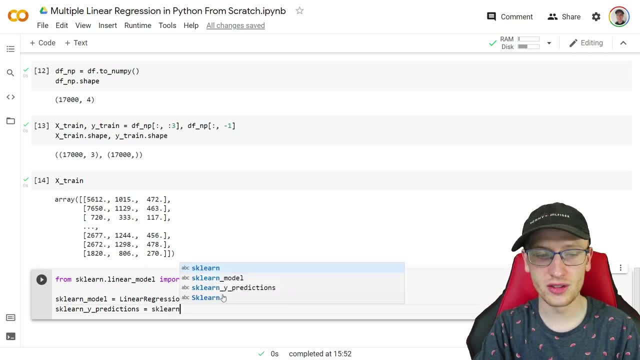 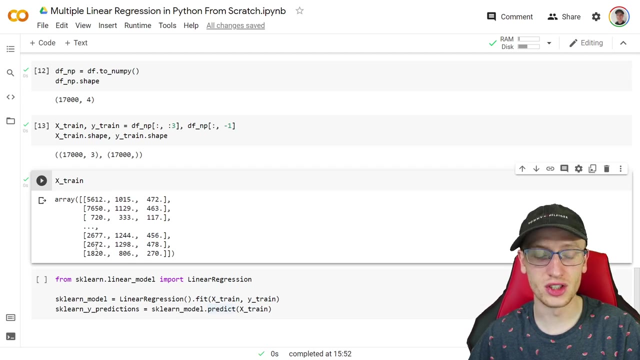 predictions is equal to. I just wrote two equals: sklearn model, dot predict with x train. Okay, so we get. we get its associated predictions after we fit it. So this is training the model, it's, it's finding the best parameters, the best slopes for each of these different, each of these different variables. 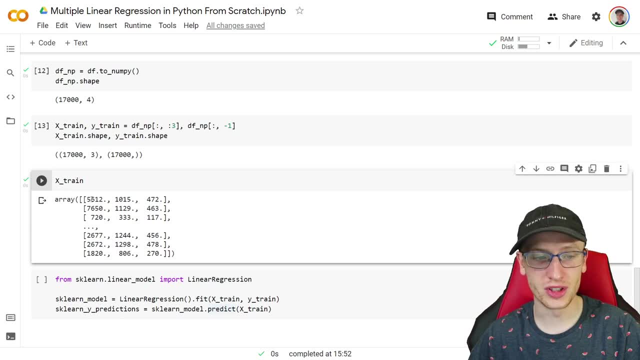 we'll find actually an intercept term- and alpha. we'll find the best beta one, a beta two, a beta three And that's just what I'm choosing to call them. you could call them other names, but that's where we usually call them, And sometimes you use beta not instead of alpha. 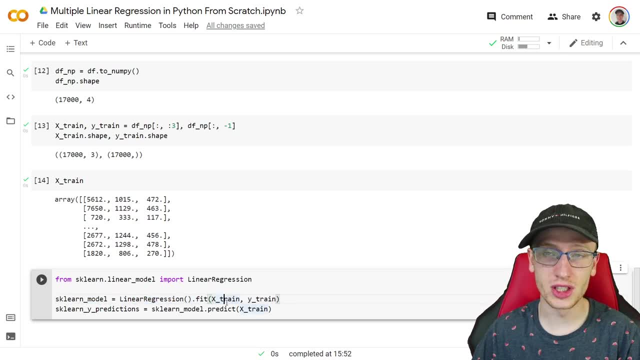 but don't worry about that. We train the model, we give it the data, So input matrix, what it maps to the outputs, we get our predictions where we actually call: predict on the training matrix which says for each of those, for each of these points, so for this, this point, these three, 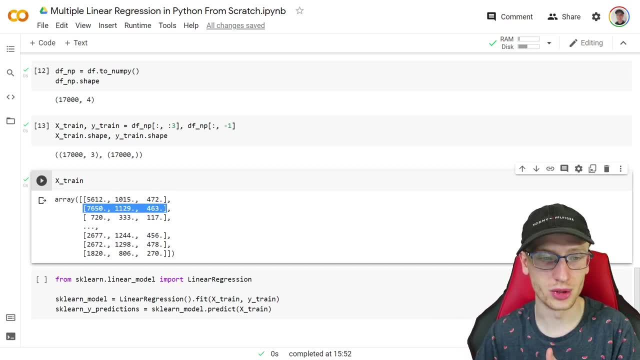 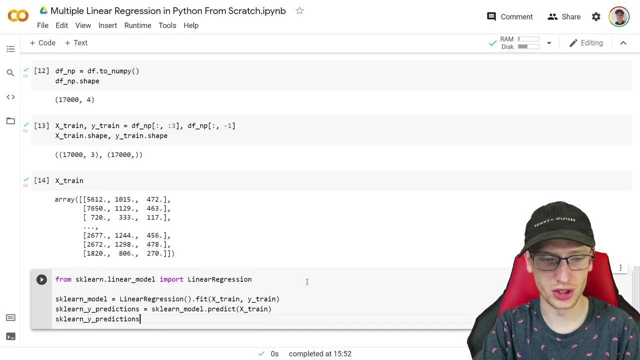 inputs. what is the prediction for these three? What is the prediction for these three? What's the prediction? So we should have 17,000 results, And so we see if we have sklearn y predictions. dot shape: it's a numpy matrix or numpy array, this time just a vector. Vector means just a. 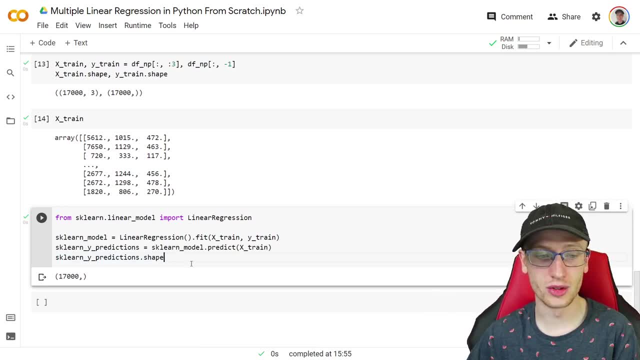 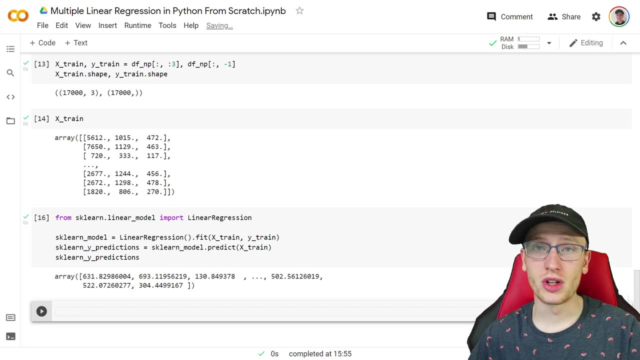 long list of information, So 17,000 values. okay, we have 70,000 predictions And I can do this again safely. Here are actual predictions And what we talked about last time and I'll go over the idea again, But basically, 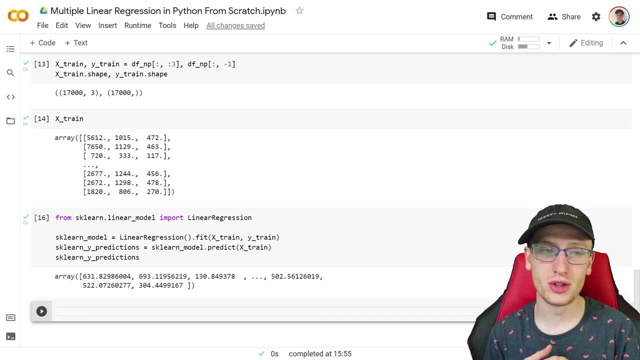 we need some way to measure error And I'm not going to write our measure or error measuring functions Like we did last time. I'm just going to import them for you, Or we have an. actually I'm Yeah, I'll show I'm for both again. So from sklearn dot metrics and I'll actually let you. 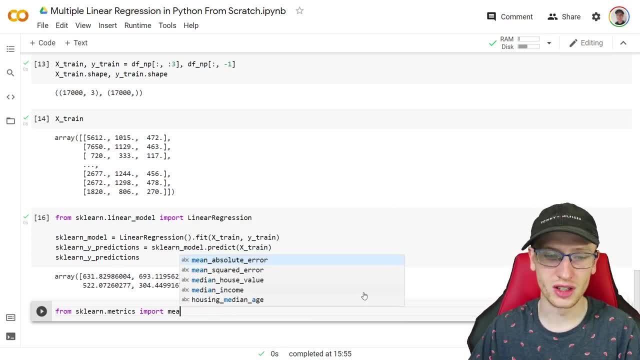 see there's going to be a long list here. we can see. well, actually it's not showing you the right thing, So nevermind. But we're going to import to mate to two metrics, which is mean, absolute error. mean means average. So, on average, what's happening? 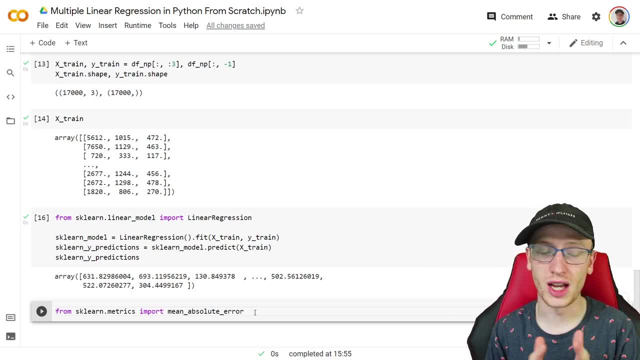 absolute error means either direction. So like absolute value, it means on average, how wrong is our model? How much are we off in the same units that the actual prediction or variable is in? so bedrooms will import mean absolute error And although we don't often or 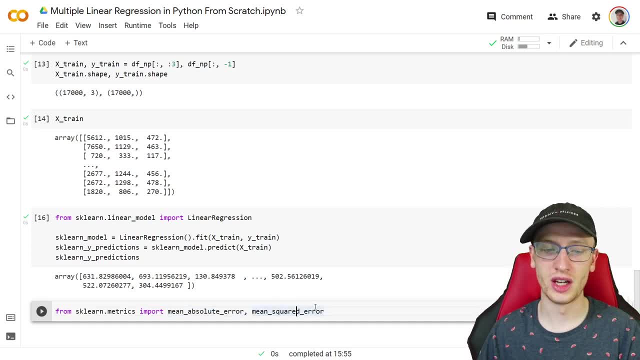 don't always use mean squared error, which is the same thing, but how? how off is it squared? this is generally what is being optimized under the hood, And we'll actually go to see that, since we're implementing it from scratch. So we can ask: what is the mean absolute error of we'll. 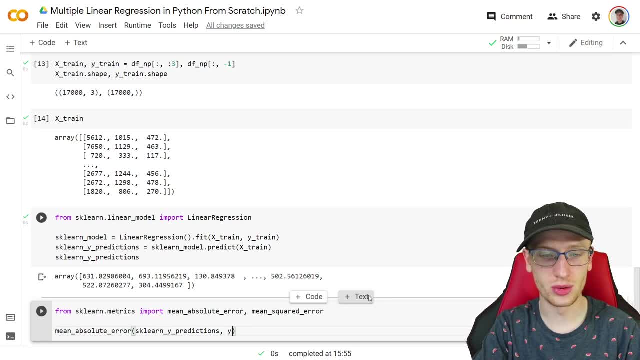 say sklearn y predictions and compare that to the actual y train. that is our outputs. So these are our observed actual y outputs, These are our predictions. Let's see what that is. And then I'm going to copy this and just replace it with mean squared so that we can see those results too. 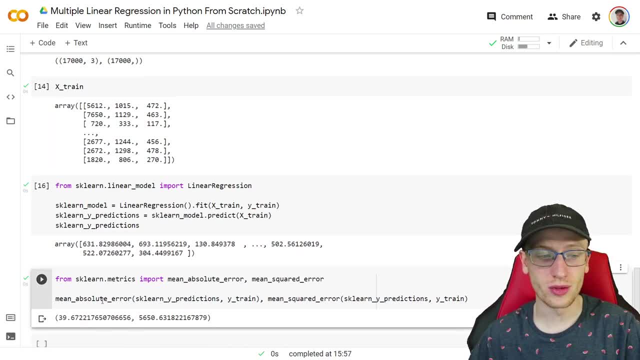 We're off by average by 40, about 40, 39.67 bedrooms and squared or off by average, squared by 5650.. Again, less interpretable, kind of weird. This is what's the mean squared error is what's being optimized. 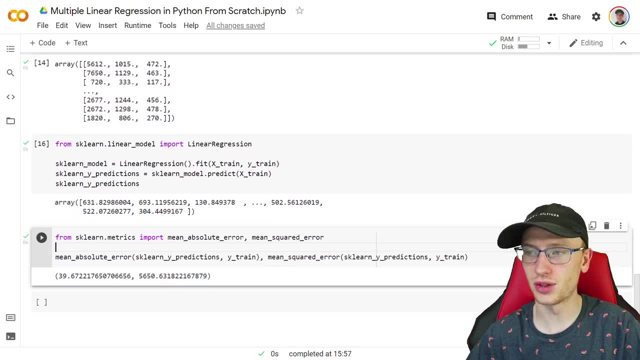 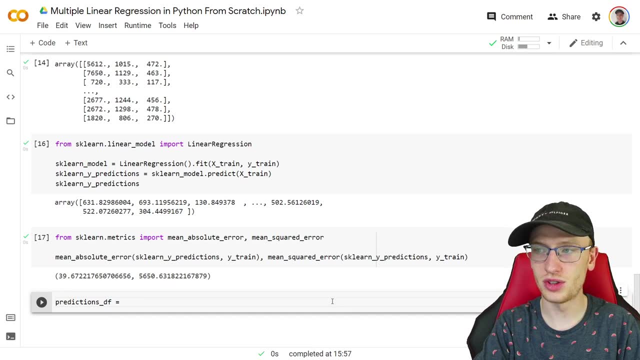 because it's easier to optimize that function than mean absolute error function. Now, like we did last time, we'll do the predictions DF. predictions DF is equal to PD dot data frame. So I'm just making a data frame from scratch And actually 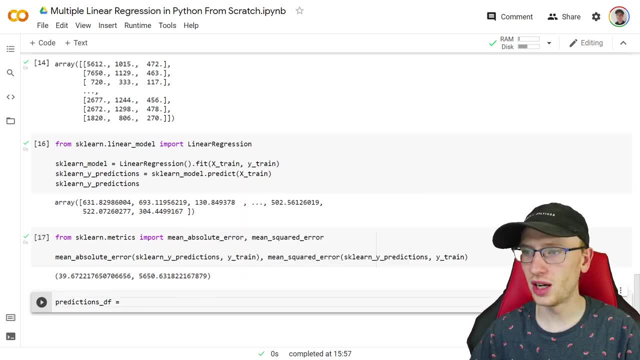 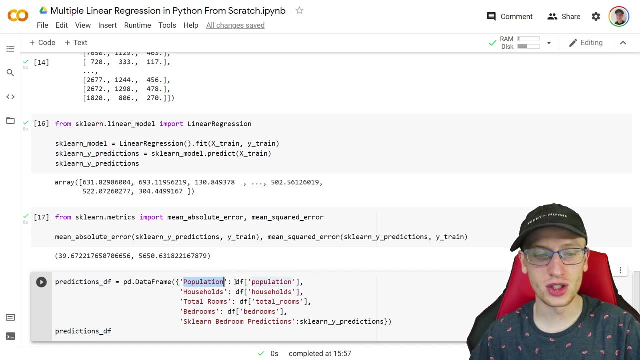 I see there's really no reason to type this out for you. I would like to copy this because it's just a lot of typing. So, basically, predictions DF is this data frame where we have the population is the population, the households is the households. the total rooms is the total rooms. the bedrooms is 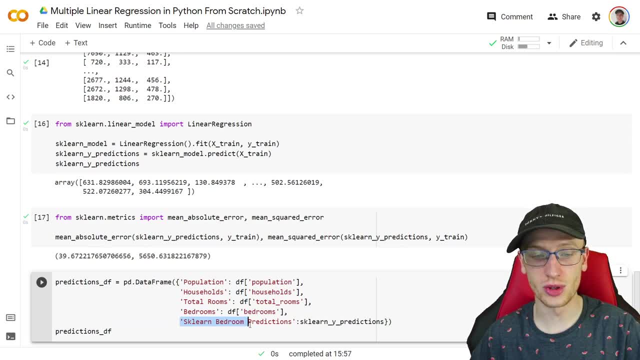 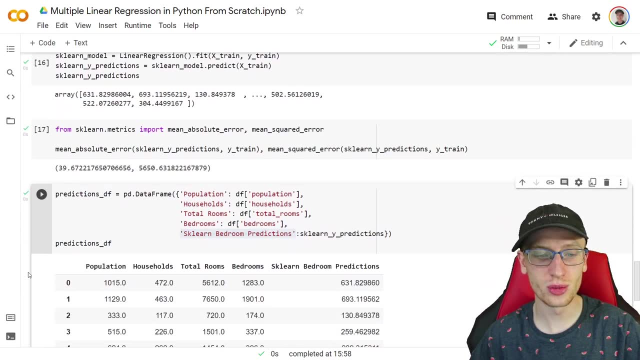 the bedrooms. that's our y variable. And so here the last two columns. this one is this last column. here is sklearn bedroom predictions And sklearn y predictions. I call it the same thing, So this should work. Basically. what we have here is, for each of these, this is our inputs. 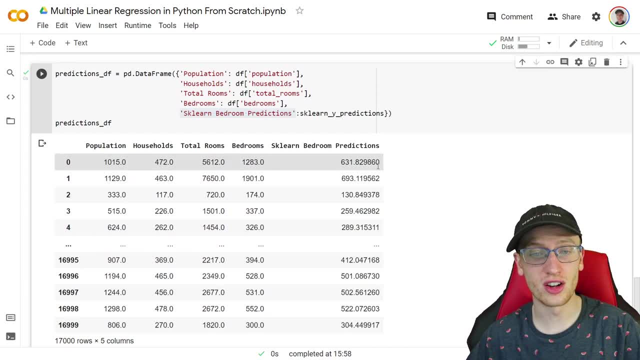 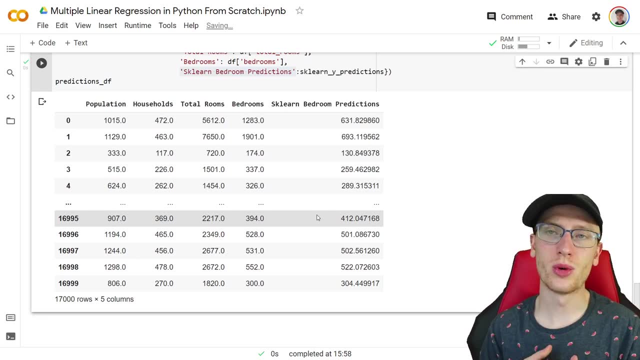 this is the observed output And this is our prediction. you can see, we're off by a lot there at the beginning, but we get a lot better near the end and also in the middle. Okay, And now, what we did before is basically plot our line where we had, okay, our input on the x axis in our output. 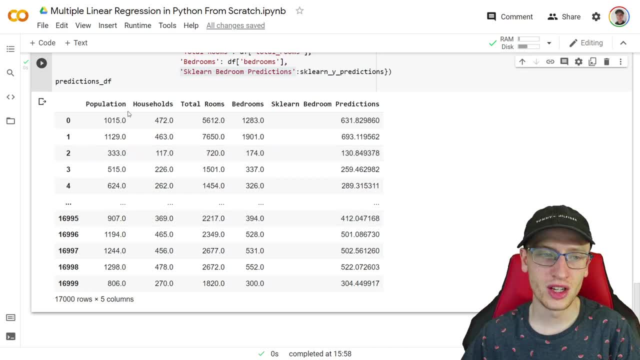 on the y axis. it's not so easy anymore, because our input is actually three variables. each thing we're predicting is with 123 different values. okay, So to actually plot this properly, you would need one axis going this way, another axis going that way, another axis going up, and then I guess that 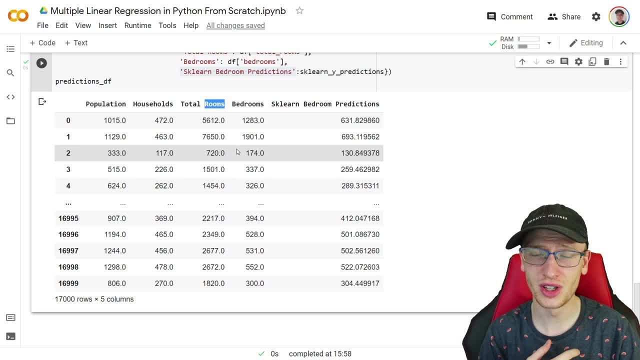 would be your three And then you could choose like a color or some sort of other way to represent the fourth dimension there. But it's a little bit confusing. you can see I'm talking a little bit weird And more generically. if you have many more columns, then there would be really no way. 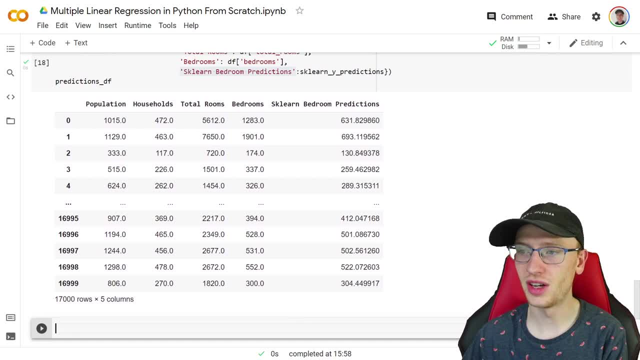 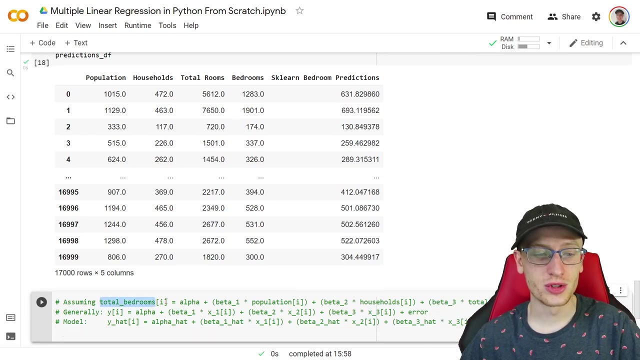 to plot this in a valid way. So we're not going to worry about plotting that data at all, really. So what we're doing is we're going to basically just copy this in here to read this out to you. we're going to implement this from scratch. Now we're assuming that total bedroom sub i. 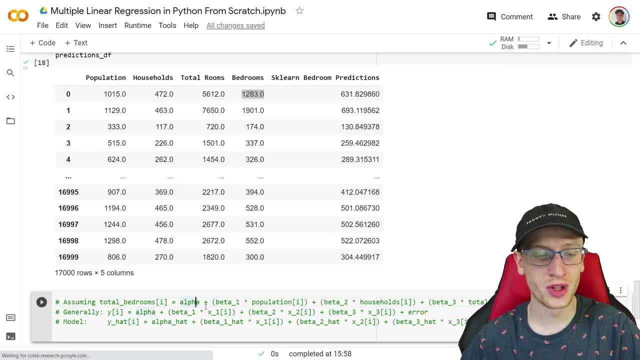 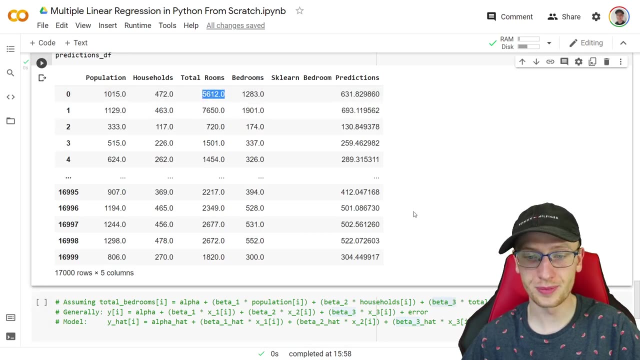 so the i total bedrooms value. whatever this is bedrooms, this is equal to alpha plus some slope beta one times the associated population value plus beta two times the households value. households i plus beta three. so my third slope times total rooms plus an error. 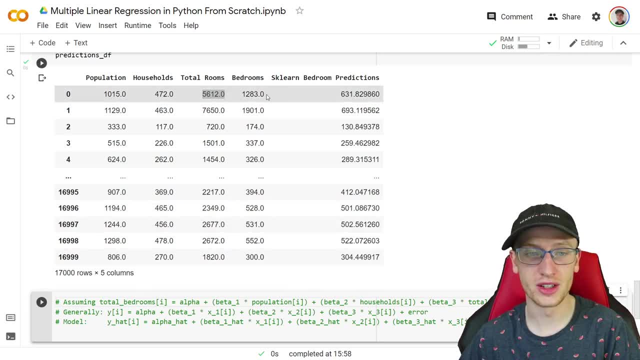 okay, that's, that's what we're assuming- that total bedroom sub i is actually equal to remember. there's going to be some extra error there, And so I said plus error. but we don't actually want to model in the air when we're trying to make a function that predicts it. well then, we don't really want to. 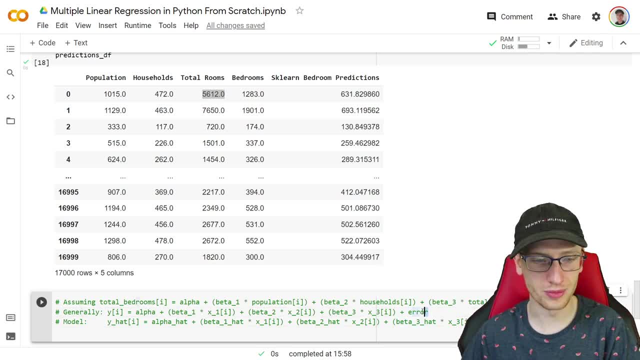 to have that included. So what we want instead? well, this is generally. I just wrote this generally as the output basically just changing the population and households and total rooms until bedrooms into, into into like just x's and y's. So the associated inputs are just ordered for x1,, x2, x3.. And the 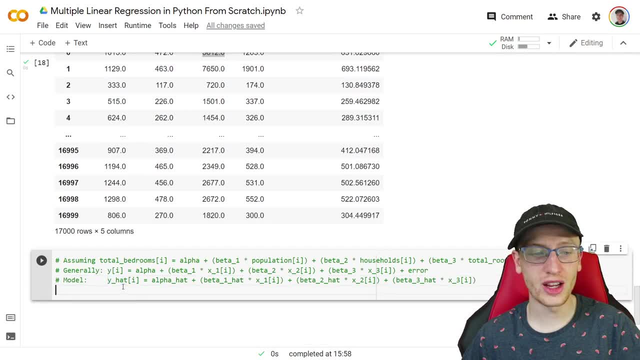 output is going to be y. Now our model is y hat sub i is equal to alpha hat. So I'm writing hats here because we're basically trying to estimate these things. we're trying to find, okay, what's a nice estimate of beta one. So we'll try to find beta one hat, what's an estimate of alpha? 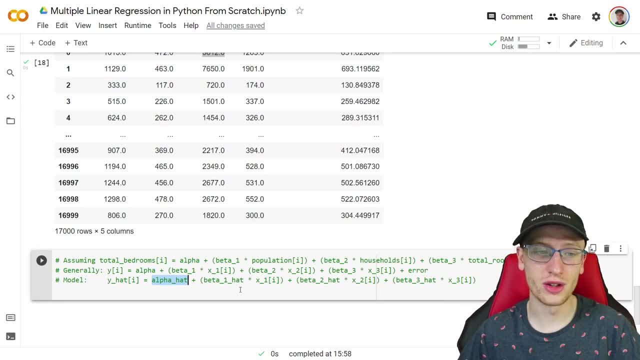 alpha hat, and alpha hat is our alpha itself, is basically our y intercept: alpha out, alpha out, alpha out. So we're going to be addingかった alpha out on these inputs, alphabets, oah, alpha hat, And so if we think about this property as some value, that'll help us. 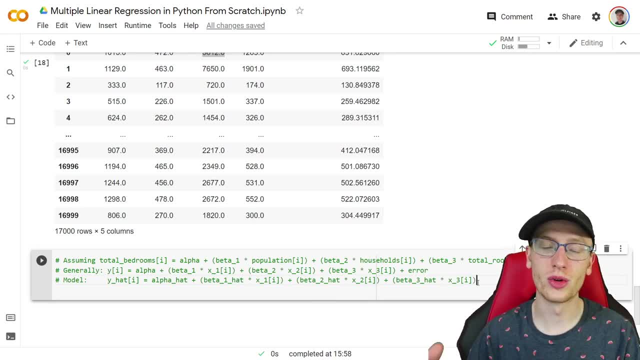 out and the other ones are slopes associated with these input variables. Okay, So that's what we're assuming our model is. Note again: there's no error at the end here. we're not going to assume in our model, actually help it predict with some random error. We're just we're going to. 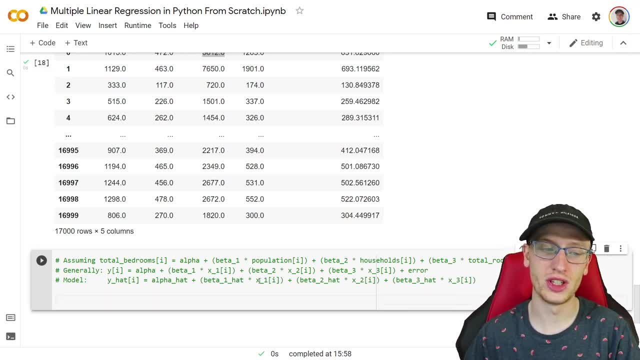 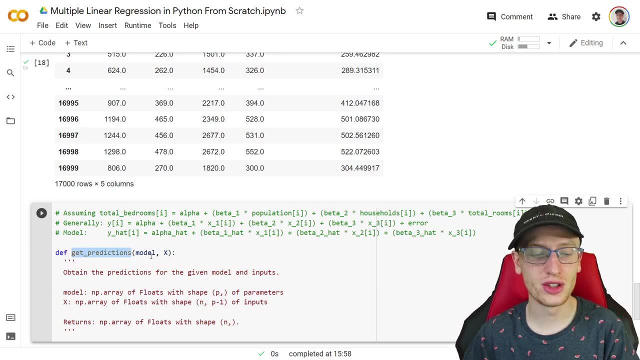 predict with this function, this line. So we're going to write this function together which is getting predictions, given some associated. we'll try to make, define, get predictions with the model and x and, if you're with us, last time we had a model as a dictionary when we we asked what alpha hat and beta hat was, but now we have. 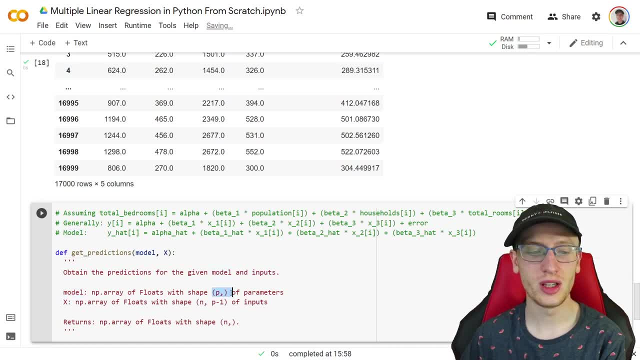 just our model is going to be p parameters. it's going to be just this list and not a dictionary of: the first value is alpha alpha hat. second value is beta one hat. third value is beta two hat and in total we have p parameters. now x is this matrix. it's a numpy array, so like a table. 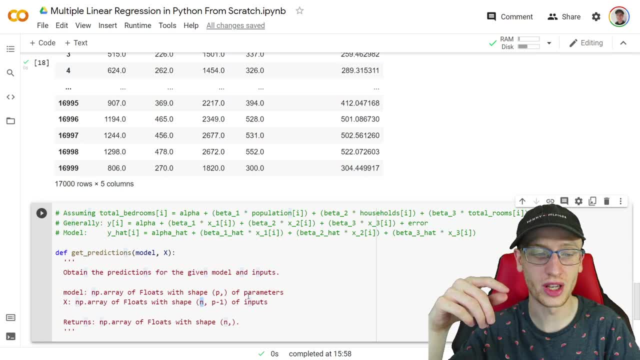 floats with the shape n. so that's how many rows we have, how many data points we have, and by p minus one of inputs. why is this weird and why is this annoying that i have to write it like this? well, i do because if we have a model- say that a model is p parameters- then our actual 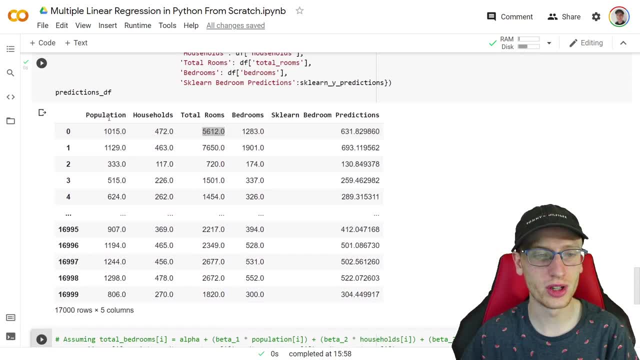 input matrix how many columns we have. if you remember, here our model is alpha, so you can pretty much just pretend that alpha is here alpha plus something beta. one times this plus beta, two times this plus beta, three times this, p would be four. we'd have four parameters and the number 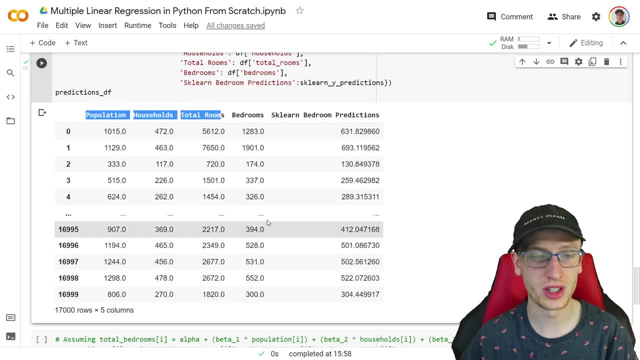 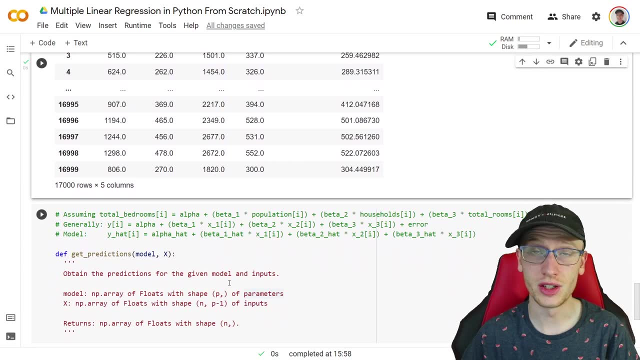 of columns that we have for our input. this would be. this would look like our x matrix here. this thing, this has three columns, whereas our number of parameters is four. so parameters is p generally and number of p, p minus one is the number of input variables that we have and we just want. 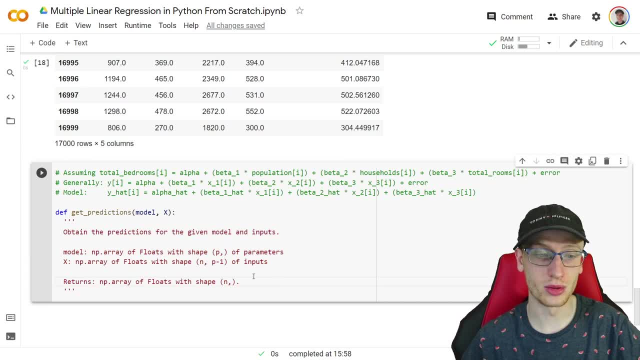 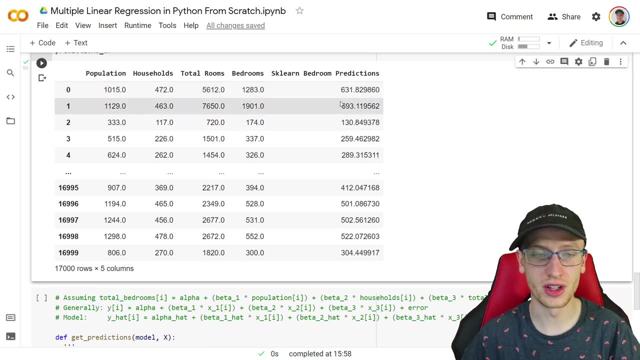 to return our associated uh outputs. okay, so, for each row, we want that matched up for each of these rows here, we want that matched up with a big vector, not not the whole thing, but we want this matrix to be associated with some vector to return some vector of predictions. okay, so, like we did before, 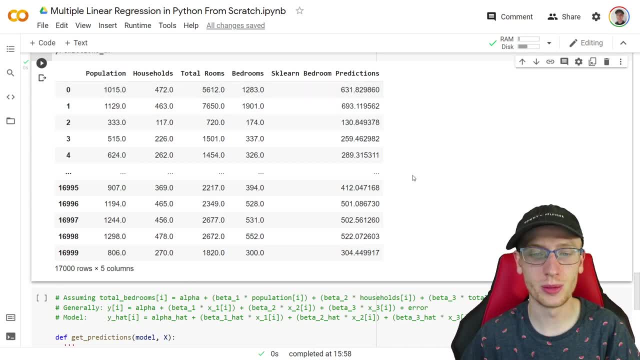 it was this big long thing. this big matrix is x and we want to be able to produce this vector y. sorry, i said that a little bit badly the first time. hopefully that made sense the second time. so we want to be able to produce this vector y and we want to be able to produce this vector y. 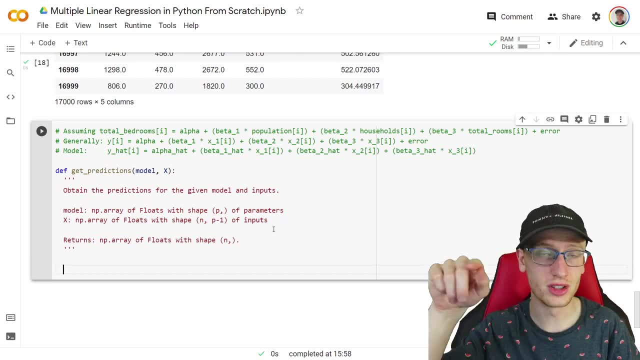 so we want to get our predictions, given our model and our output. where our model is this vector of information? actually, i should draw a vertical line, as i'll show you shortly, and x is our matrix here. so i am going to go over to paint and draw you a picture. okay, let me try to draw you a pretty. 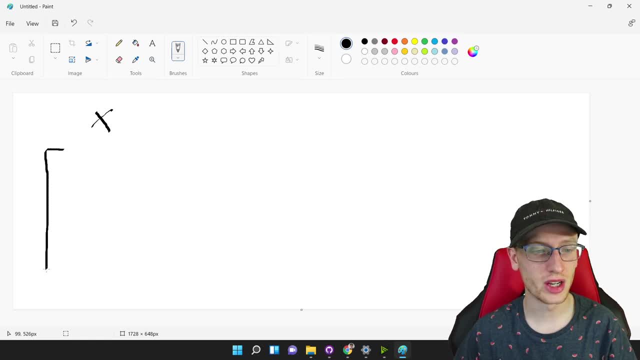 picture here. so if we have our input, matrix x, where we have, how many rows do we have? we have n of them. so like this, i'm going to say this is n, and then how many columns do we have? we have p minus one. i'm going to leave a vertical blank here at the beginning and you'll see why shortly. 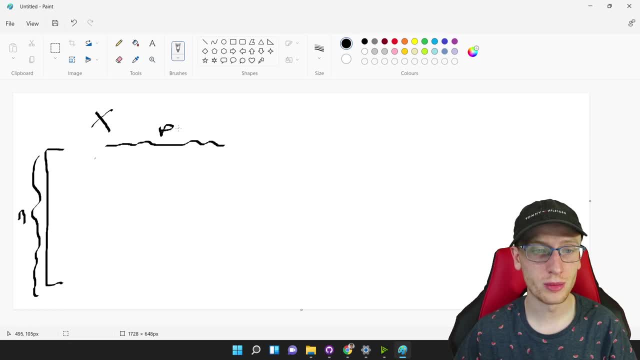 so going across like this, we have p minus one items, so this should be- i'll write it as x one. so this is the first row. this first index indicates the row. the second one indicates the column. so this is x one and it's going to be the first one. okay, so the first variable, the first. 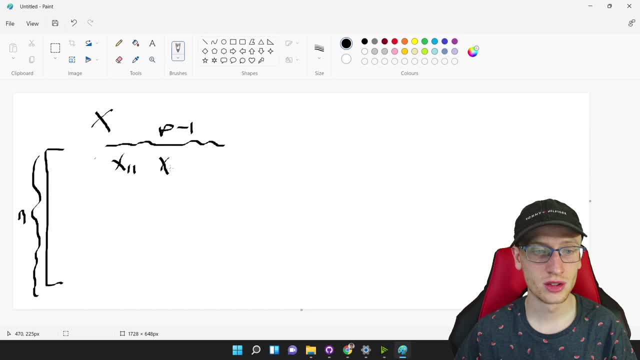 first row, this is going to be x one, two, so the first row, but the second column, and this goes all x one p minus one. okay, so x one. this one is always the beginning because we're in the first row, and the second item is the column x one one, x one, two x one p minus one. now, if i fill this, basically if i 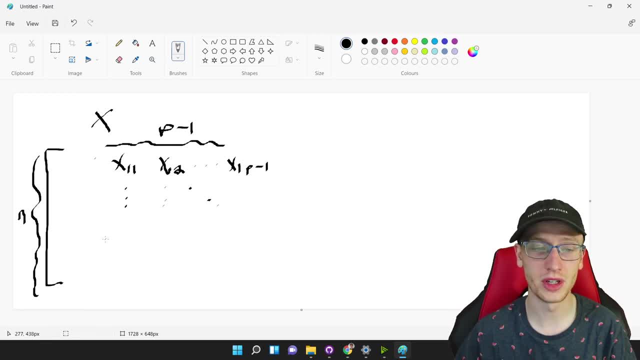 fill it like this. it's just a shorthand way to say like: however many we have, this should go all the way down until this is x n one. okay, so it's the first column, so this stays the same. this is one, but this is the row. so x n one. this is x one one. this is x n one. this is. 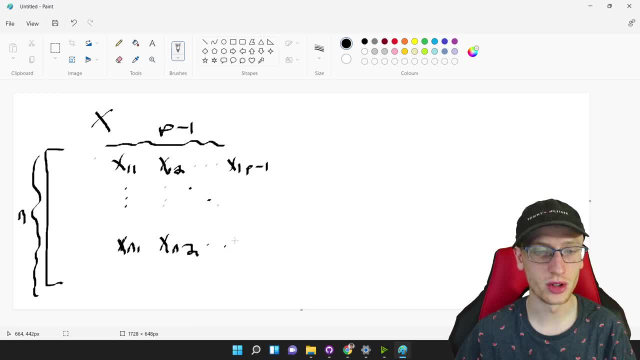 going to be x, n, two, and this is going to go all the way up until this is. what value is this? this should be. well, it's the nth row and it's the piece or p minus 1th column. so this is x- n, and then the. 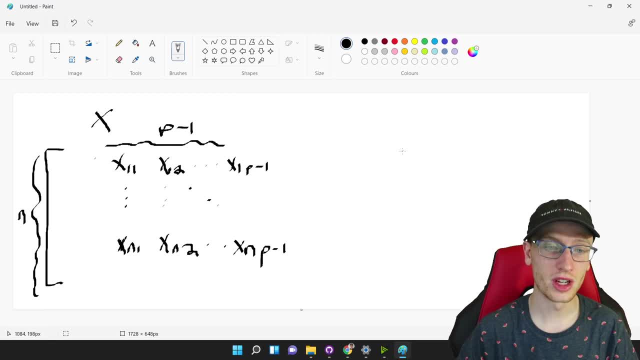 second one is p minus 1. okay, so it's kind of weird written like that and i apologize for it being weird, it's, is it? this is a tiny math lesson and i hope this makes sense for you all. okay, so, if we're sense. So this is our input matrix. It looks like this: We have our parameter, basically our model. 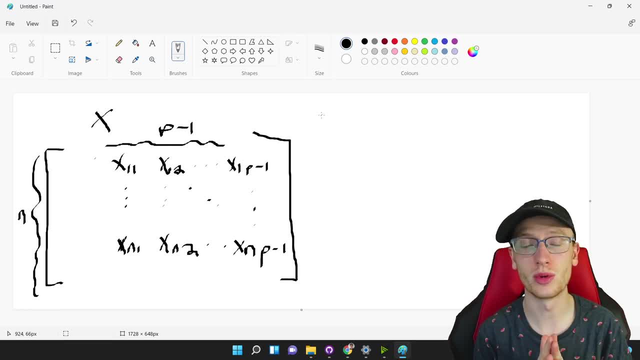 which is a bunch of parameters. It's just a bunch of values we're trying to learn. We want to figure out these parameters. We're not worrying about learning them yet, though This is just assuming that we have them- given some particular parameters, which is, we'll say, alpha, and actually how you 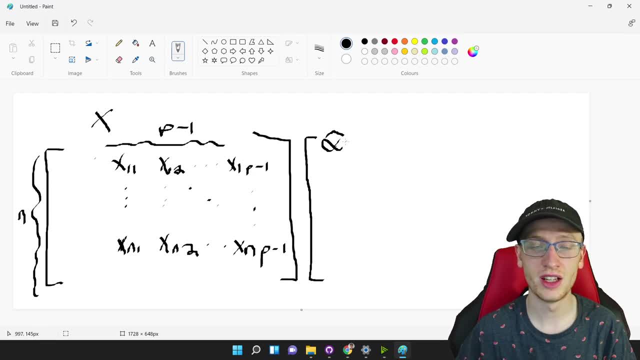 would draw it. I'll draw it with hats. So this is why I'm saying hat. This is alpha hat, which is our basically intercept term, Beta one hat, which is our slope, associated with the first column. So it's always associated with these variables, and we'll see why shortly. And this goes all the way. 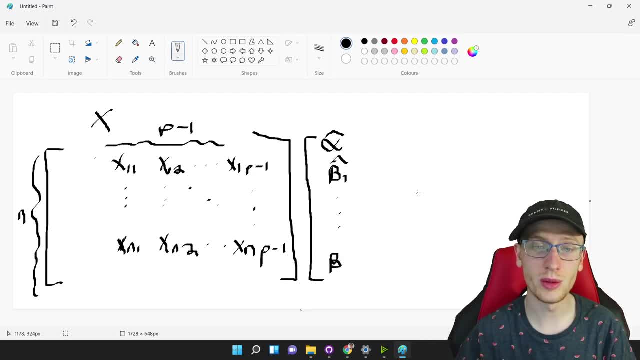 down until what is this value? If we have p parameters- total, this is our p parameters- then this should be beta hat p minus one, So there's p minus. sorry about that. p minus one things here. plus one is there should be p things. So it doesn't really match up right now because we 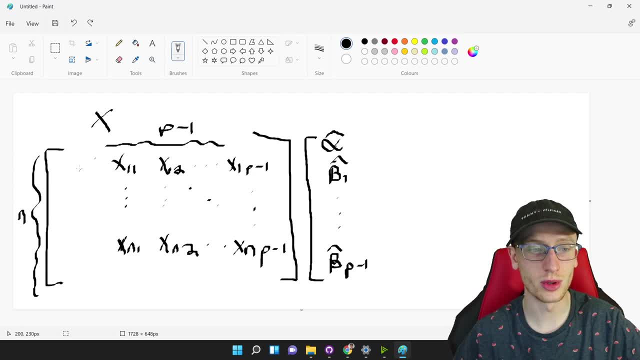 have p things here. So we have p things here, plus one is there should be p things. So it doesn't match up right now because we have p things here. So it doesn't really match up right now because we have p things here and we have p minus one things this way. So we draw ones here. Let's go. 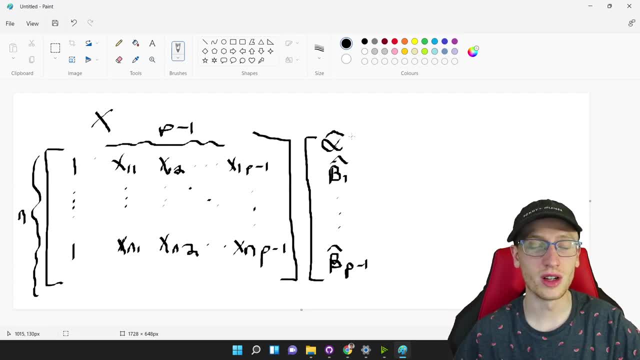 this whole first column is ones. So that we'll see why. for two reasons. The main one is because this whole thing now across, this whole thing, is p dimensional, There's p things across, so that this, these two shapes match up. This is p and this is p. Okay, so what we actually want, 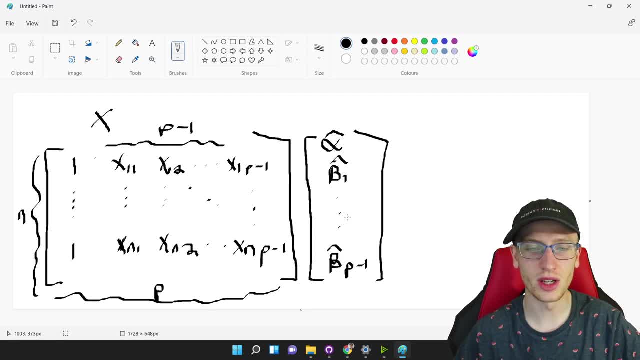 to do here is basically if you can think about stretching this thing out so that it's horizontal, So if you stretch this out so that it's alpha hat and then beta one hat, and then up until beta p, beta p minus one hat, If you stretch all this out sideways, basically think, 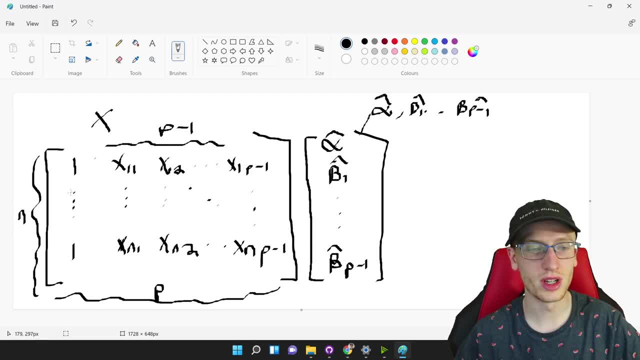 about pairing this thing up sideways with this row and then this row and then all of the rows here, so that it's always and you do multiplication where they touch. So it's alpha hat times one, which is just alpha hat plus beta one, hat times x one, one plus, if there's a two here, beta one. 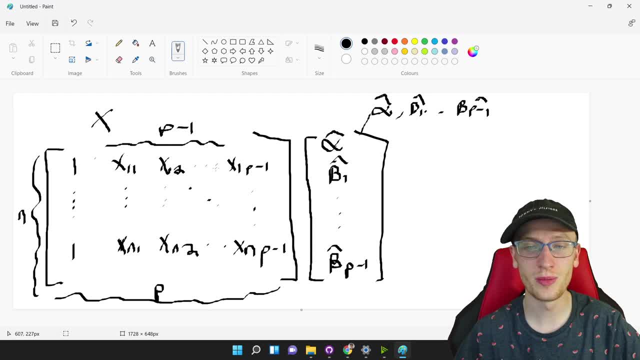 beta two, sorry, beta two. hat times x, one, two, all the way up until beta p minus one. times x one, p minus one. If that was confusing, don't worry too much about it, But basically we do, we make this. 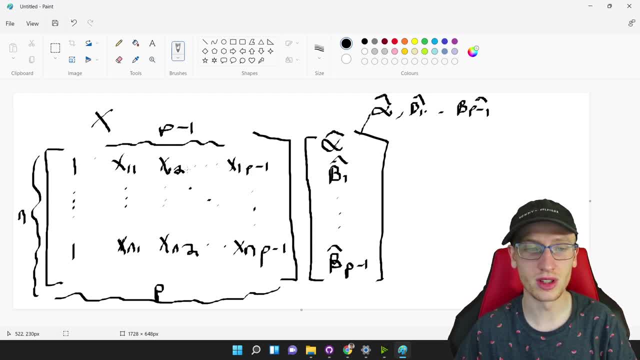 to be a pairwise multiplication with and sum it with with this vector right here. So sorry about that. that probably didn't make sense. What we do is alpha hat times this plus beta one hat times this, all the way up until beta p minus one times this, And we do the same thing. 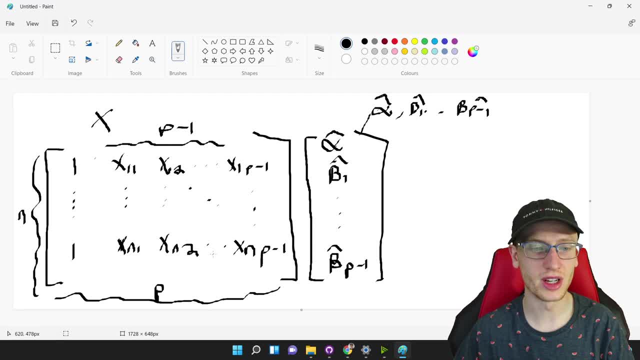 down here: alpha hat times this plus beta one hat times this plus dot dot dot, all the way up until plus beta p minus one times this value, right here. And so what that's doing is basically just converting this. if I write it like this, this is converting it to a vector where, if we do that, 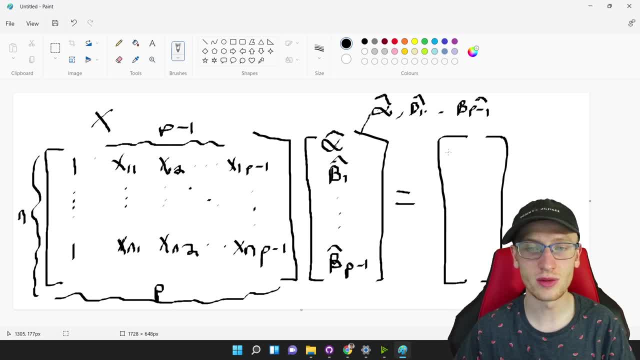 multiplication and sum. like I said, this, this value here, this would be our prediction for the first row. Okay, so we have. we have n of these things. this is going to be n dimensional. we're going to produce in n, n rows here, And so that's the first prediction because it's our linear. 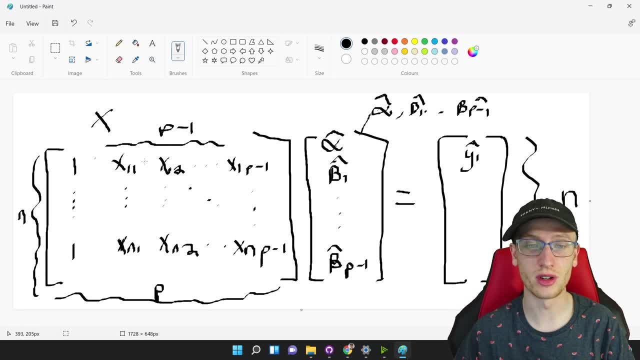 our models multiplied and added with our inputs here. that's what we're assuming the relationship is, And this goes all the way up until y n hat. So these are our, these are our associated predictions. If this part didn't make sense, do not worry about it too much. I really don't think. 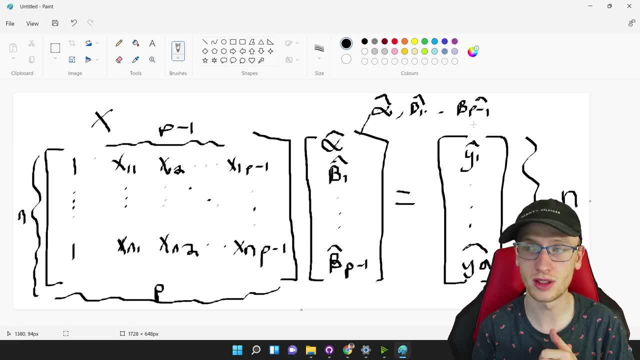 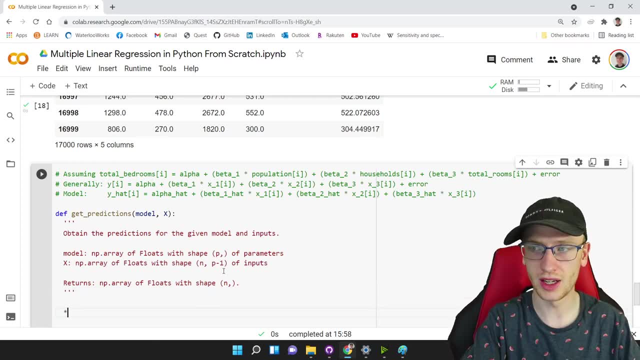 it matters too much, It's just a bit of a math lesson I wanted to throw in, if it makes, so that it could try and make sense. We are going to write this code, And so, basically, we're going to write this code, And so, basically, we can get our shape as we can do- n sorry the tuple- we can. 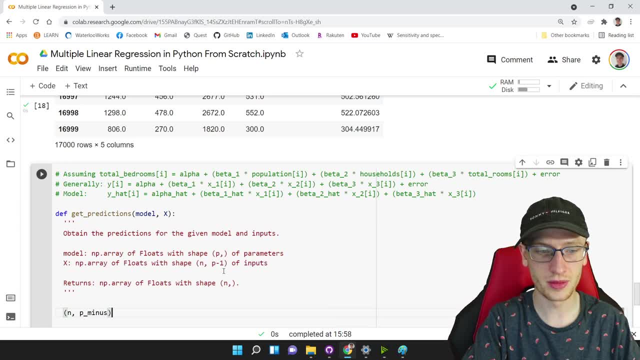 get n and it'll be p minus one. p minus one is equal to x dot shape. Okay, because that's what we said. it is x is n by p minus one, And then of course we can get: p is equal to simply whatever. 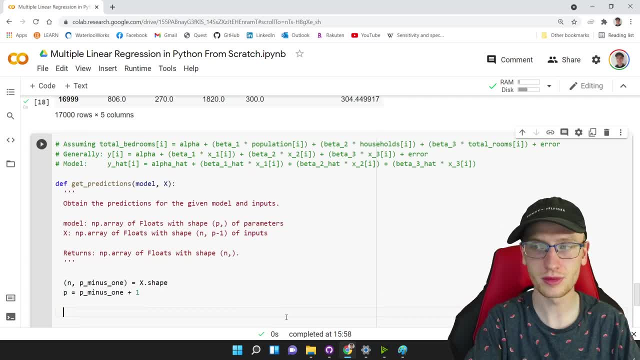 p minus one is plus one. So now that we have that as well, what we're going to do we want to add a column of ones, So that that column of ones was important to us. So we're going to say: new x is: 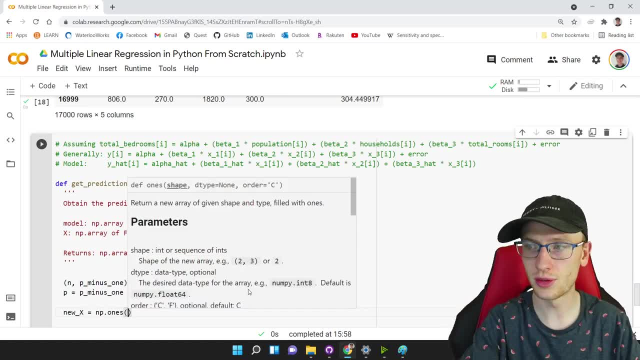 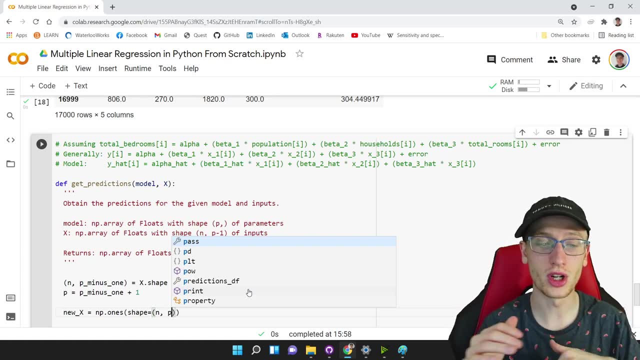 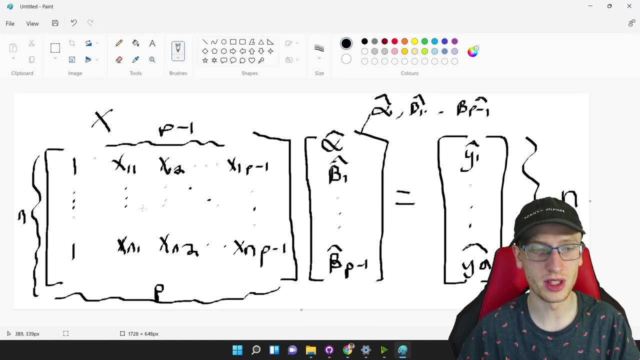 equal to the numpy dot ones, which is simply a matrix of ones where we set the shape equal to n by p. Okay, so now we have n rows and p columns, all are ones. But to actually get back, basically what I'm doing is just trying to get this actual matrix. what we have is this piece: 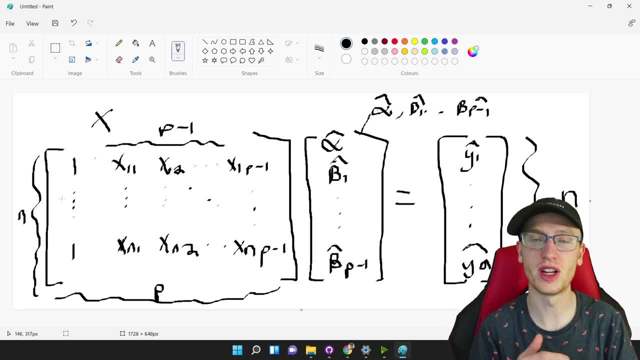 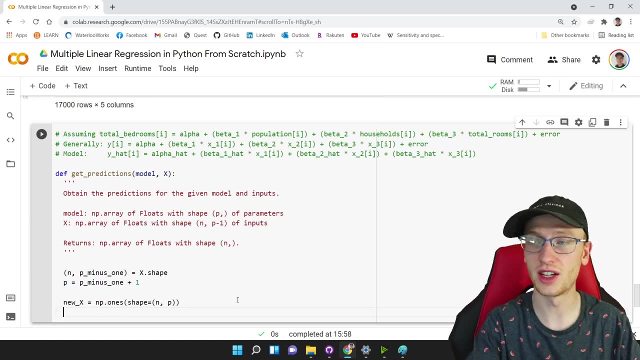 here. we don't. we just have this ones, or we're trying to add in these ones. what I just did is this whole thing so that it's ones, and then I'm going to override this particular section with the x variables. So I do that with new x. is simply this to start? it doesn't have any x in it. 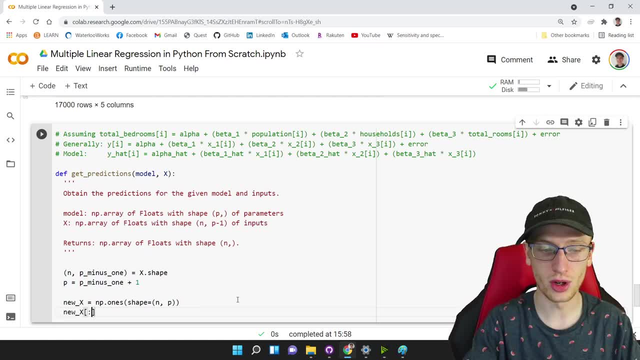 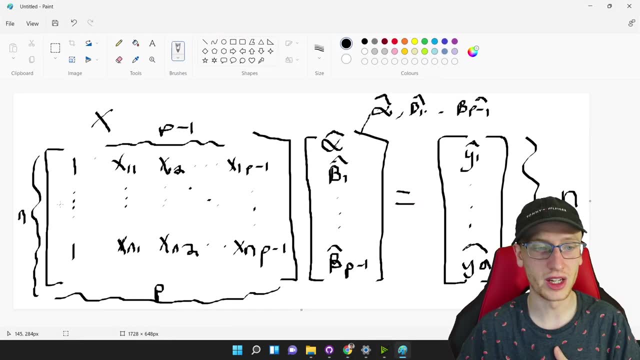 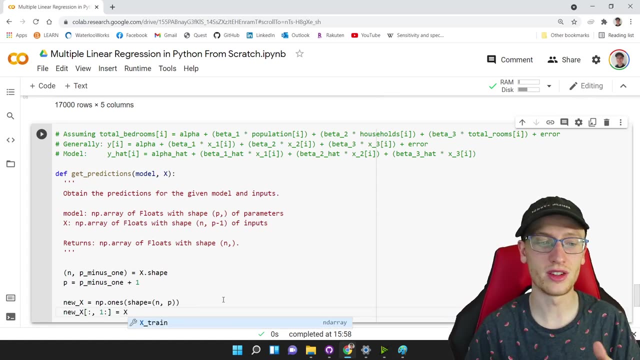 yet What we'll do is new x, new x, so all the rows and then one comma which says those last, those last columns, So anything but this first one, all of these columns here. we're going to override that and set that equal to x, So that new x now. 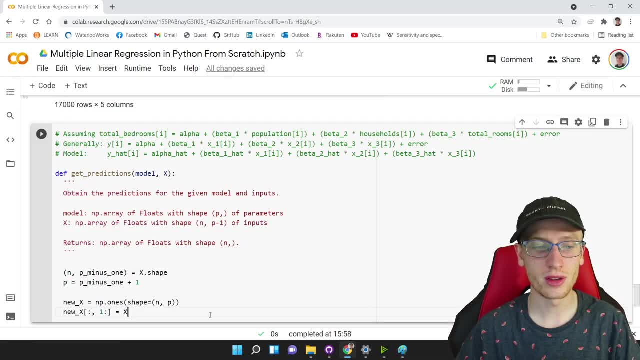 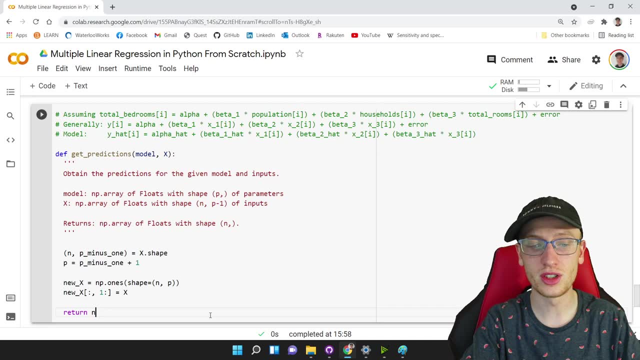 is actually that proper picture here, And then we can do the math like we just said. what it's actually called is matrix vector multiplication, And actually it's kind of a weird term in numpy, But we're going to do, make that or call that with return numpy, dot, dot of. 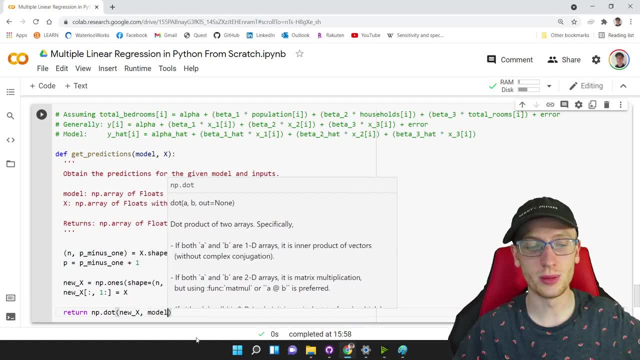 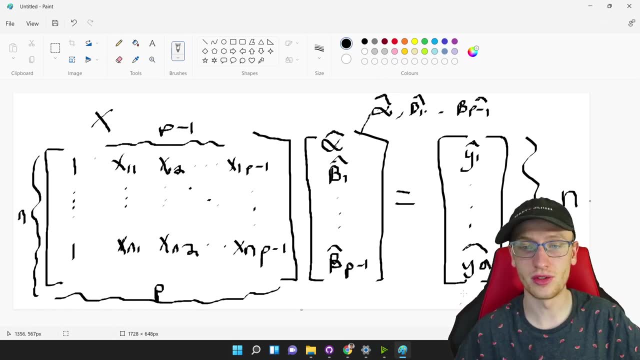 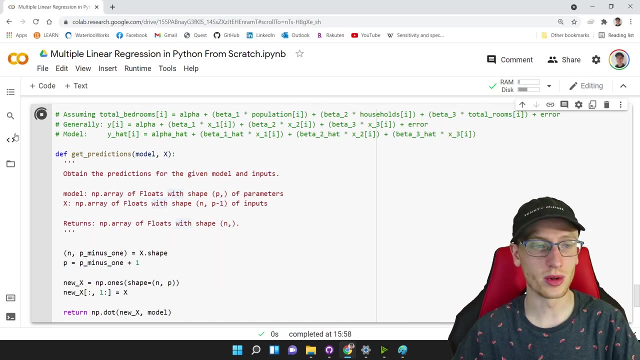 new x, new x and the model. Okay, so you can pick picture this thing as new x here And this is the model. And np dot dot will make this prediction vector so that it returns a numpy dot array of n comma. that's what it does. Okay, I will run that and we can test it with. how do we do it test? 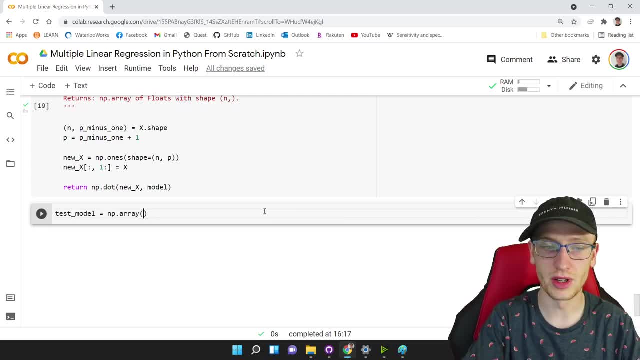 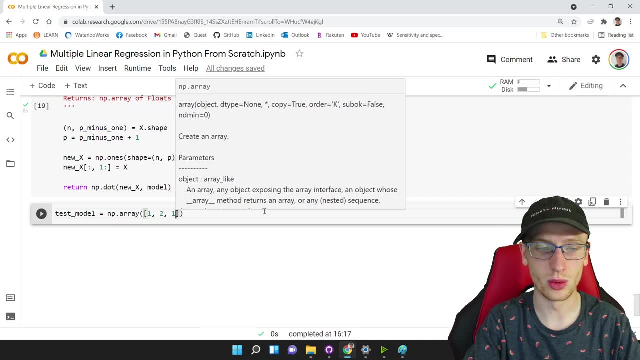 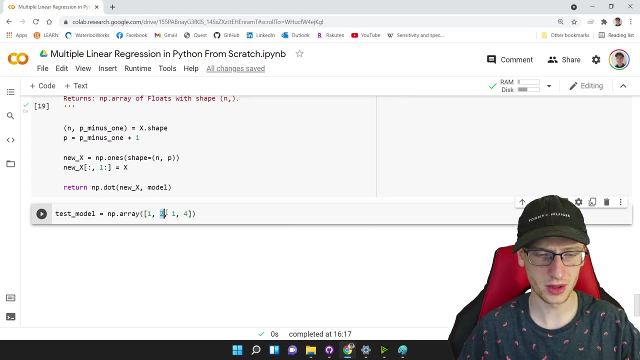 model. So just the test model is equal to numpy dot array of. we're going to make it four items to match with our particular example. So I'll just get random values: 121 and four. So that's saying alpha hat, maybe it's one, beta one hat, maybe it's two, or- Yep, sorry, Yep, that's right- Alpha hat. 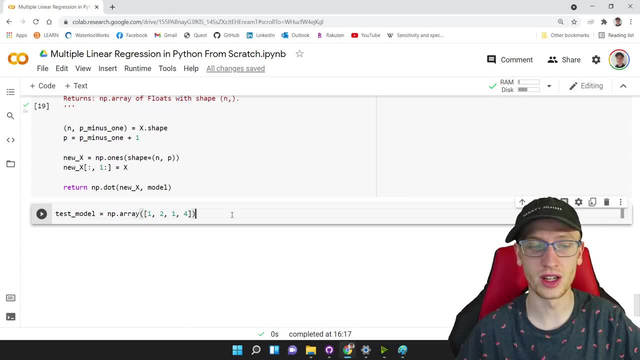 one beta one hat to beta two hat one and beta three hat. Hopefully I said that right And we can get the predictions, get the predictions with our test model. So we pass it. how do we call it? we pass it the test model And then we give it our input. 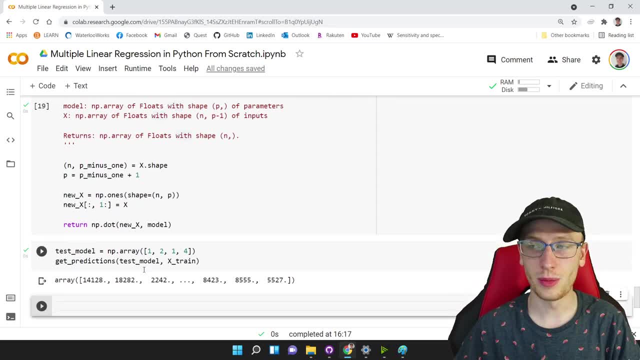 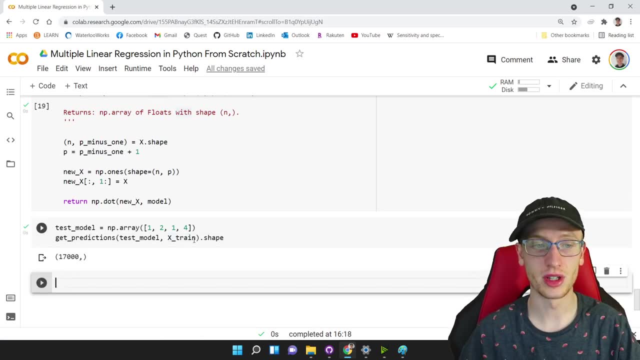 matrix, which is x train, Okay, And that makes a series of predictions with a shape, a shape of 17,000, comma, okay, so n rows. hopefully that makes sense. And so this, what this does is has predictions. 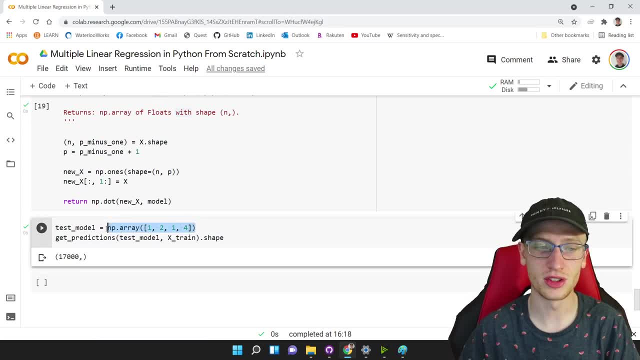 For a given model. This is just. we chose this model. It's just an arbitrary choice. It's not necessarily the best model, But it's. it's an okay model- Or actually, no, it might not be okay at all. It's just it's. it's a model. Basically, what I'll do here is add to the predictions DF what? 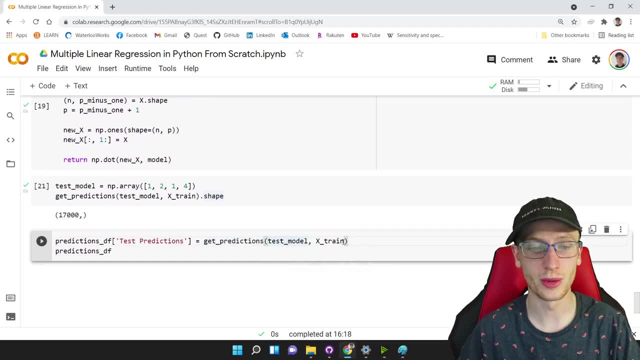 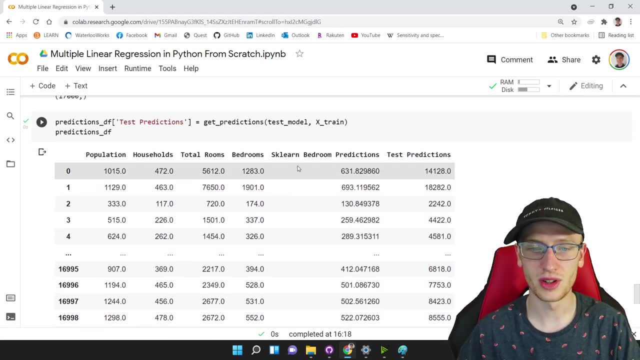 we were observing before the same thing to get predictions with the test model and x train. So that same thing here And we can look at predictions. DF is here's our predictions. Not very good, Okay. so 1283 is the actual 14,000. 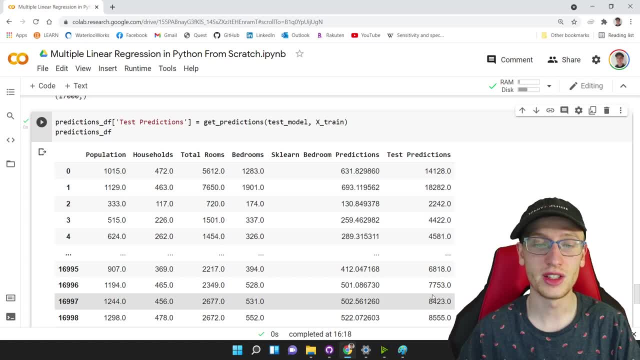 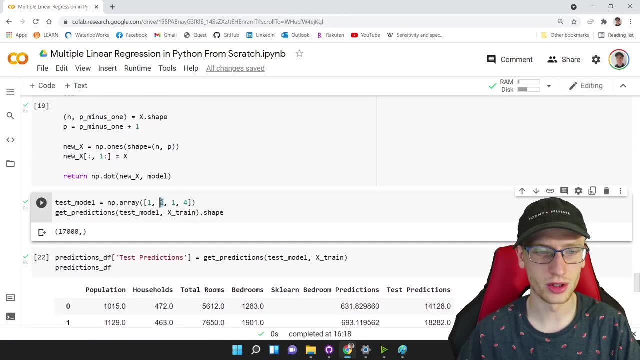 Was our prediction 531 8400.. It's really really far off, And so maybe if these values are too big here, then, you know, maybe we could make a better model with maybe saying this to one sending us to: 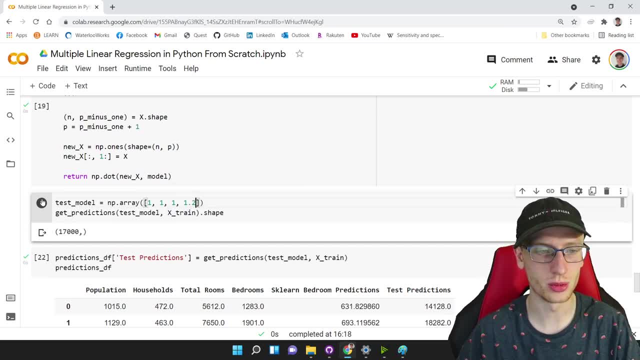 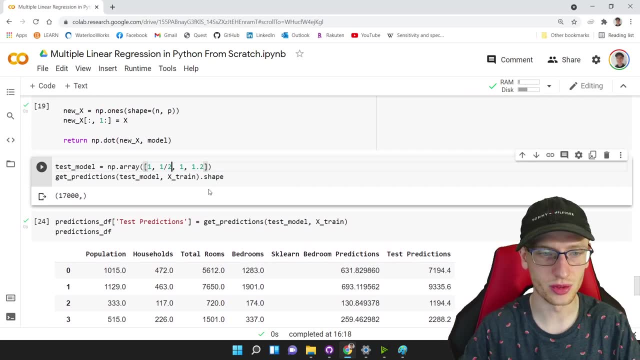 maybe, maybe, I don't know. 1.2.. These could be floats as well, So let's try that And we can see you know. clearly it got better, but it wasn't great. Maybe we'll set this to one over two. 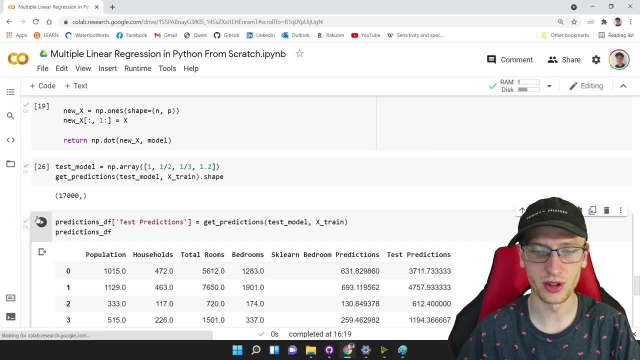 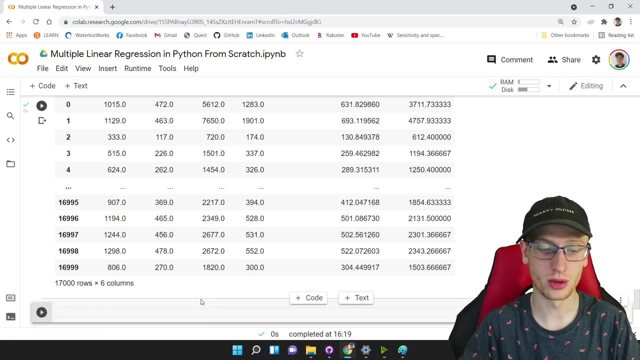 maybe one over three. I'm really just picking things to make it smaller, I don't know. Okay, and maybe it got a little bit better. It's still not great, though We can actually measure its error, So what I could be doing here. 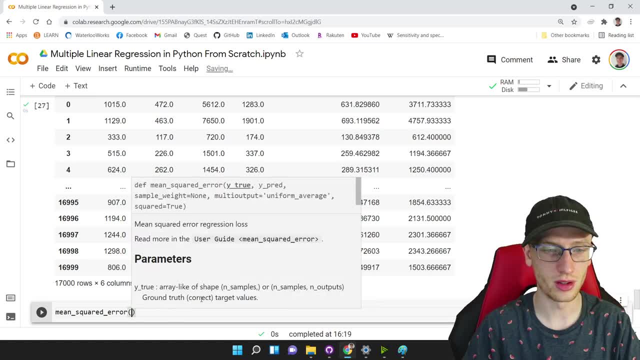 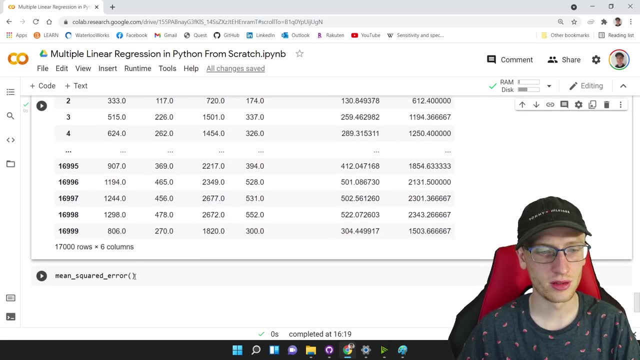 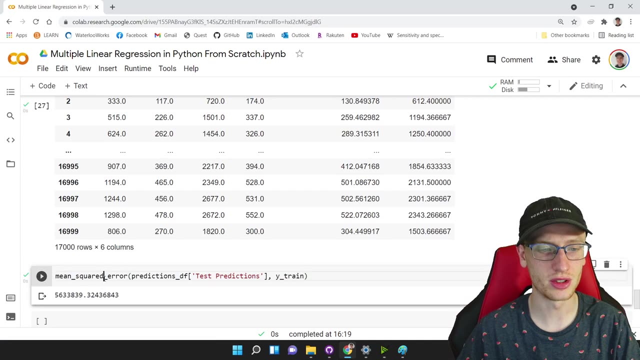 is looking at the mean, absolute error of. if we look at what is, it's grab it as this predictions, DF, sub test predictions, this column here. If we look at that and compare that to why train the actuals, then that gives us a mean. sorry, actually, I want. I want absolute, not mean squared. 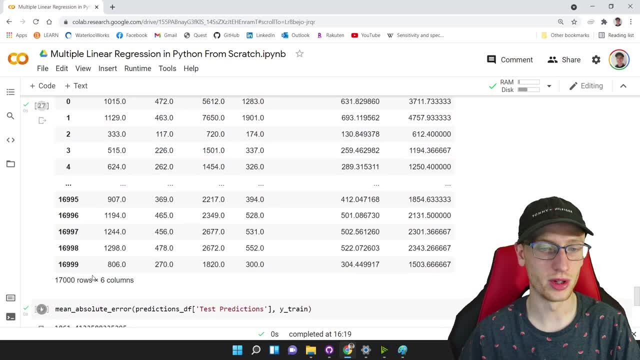 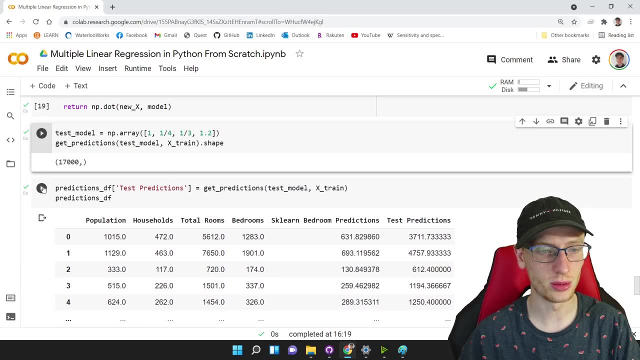 It's not so great. Mean absolute is off by 1861. Maybe I'll try to get a little bit better, And maybe this should be one over four. So can I get better than 1861?? No, that looked very, very similar, So I'm surprised at how similar that was. 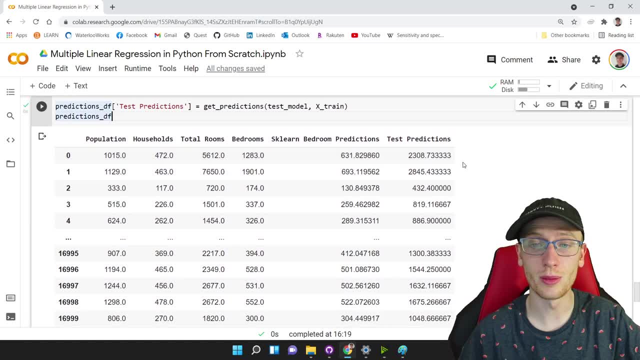 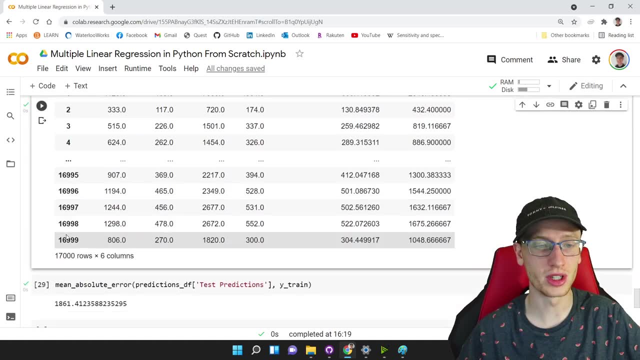 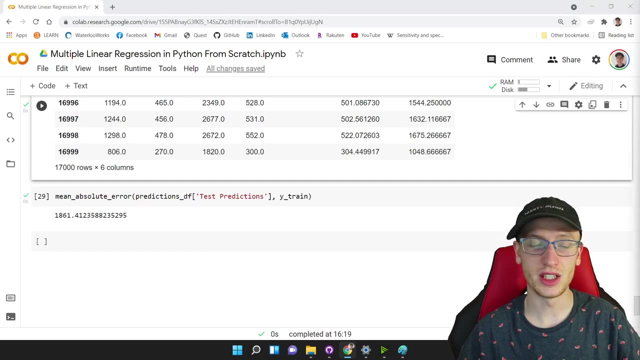 But anyways, okay. so here's our. our model makes these predictions with: with these inputs, we want to find better parameters. clearly, we want to minimize- we're going to minimize- the mean squared error function, And we do that with something that's very confusing, And I just 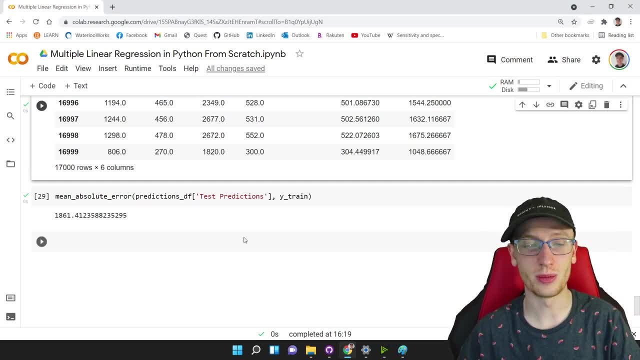 want to paste this in here, And I'm going to paste this in here And I'm going to paste this in here And I'm going to paste this function in in for you and read it, because I'll redirect you here. 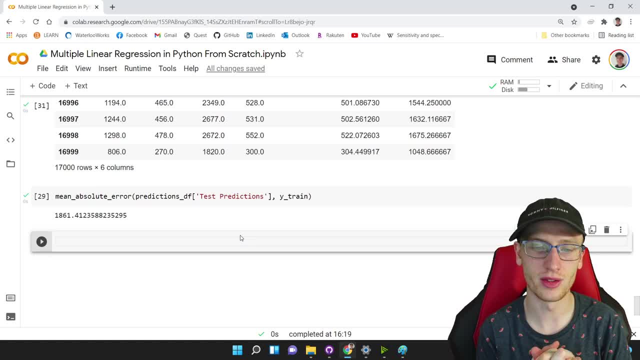 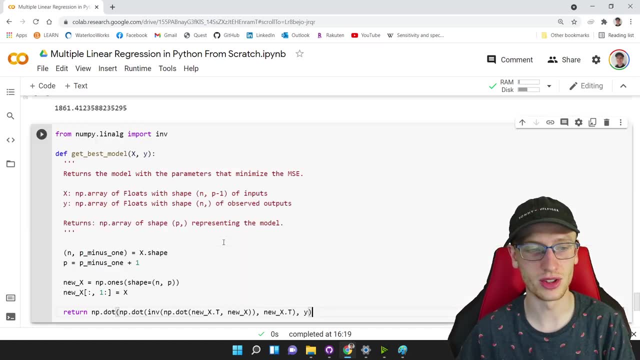 if you want to know the math, it will take a fair amount of effort, kind of like. you probably got confused with the paint picture, This this would get very, very confusing on how to do this. The important parts, and actually I'll save the implementation to not distract you from. 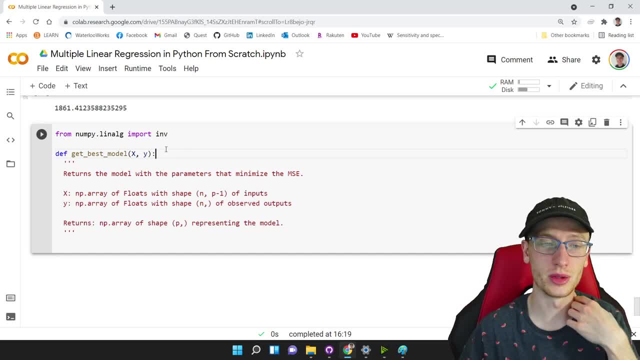 the important part just yet. we want to get the best model, which is a function- don't worry about this import- that returns the model with the parameters that best minimize the mean squared error, That minimum, that function, And so we have. x is a numpy dot array of floats with the shape of n. 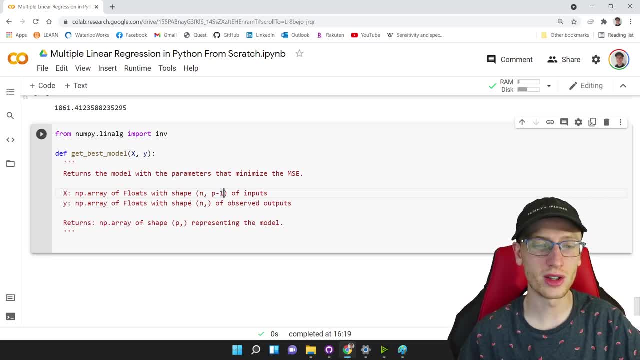 p minus one of inputs. those are inputs as before. y is the numpy array of floats with the shape n comma of observed outputs. okay, so we give it that's basically like fit, before we give it the x and the y, And it returns shape. it returns a little bit of a different 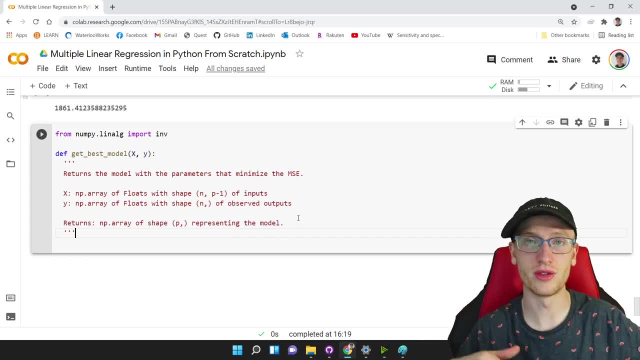 object than SK learn does. this is just a vector of values and then pi array of parameters representing our model. It returns the best parameters that will minimize the MSE, assuming it's a linear calculation, linear formula. So how do we do that? It turns out we. 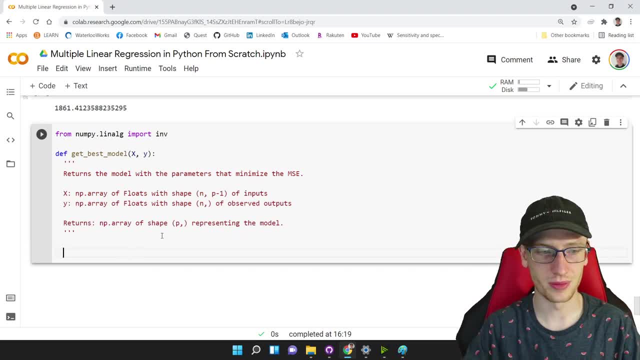 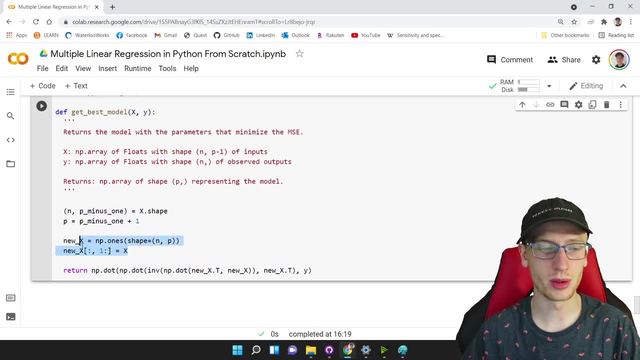 do it like this and I'll just copy it in for you. Here you go. So this is the same thing as before. we get n and p, we make our matrix in the exact same way, so that new x is that paint picture as: 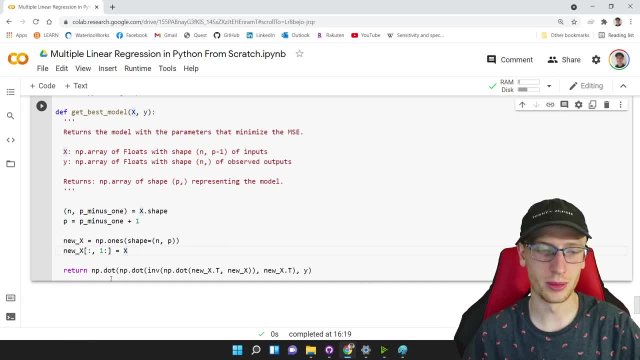 before, and then we do the numpy dot dot of the numpy dot dot of the inverse, that's the numpy dot lenounce dot inverse of the new x, t. So basically this is a formula that I've had memorized since it came up in my stats class. If you're interested in this, definitely take an. 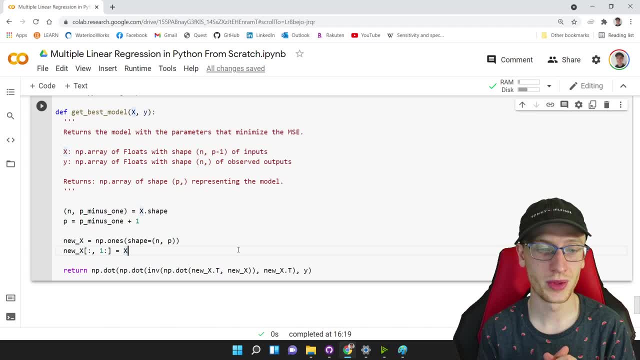 undergraduate statistics course in linear regression and basically the formula is: x transpose x, inverse x transpose y. If you don't already, you probably don't know what I said in, unless you already know what this is, and then I wouldn't really be watching this video, if that. 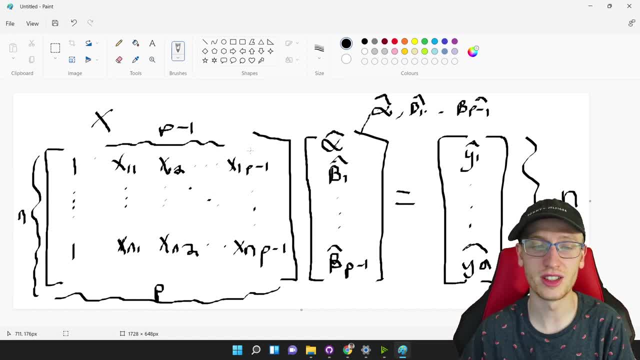 were true. So basically, transpose is a. what I said is a certain operation on a matrix which is this, the inverse. there's an idea of the inverse of a matrix. it's also a matrix and you can do matrix multiplication as well. This is matrix vector multiplication. you can also multiply. 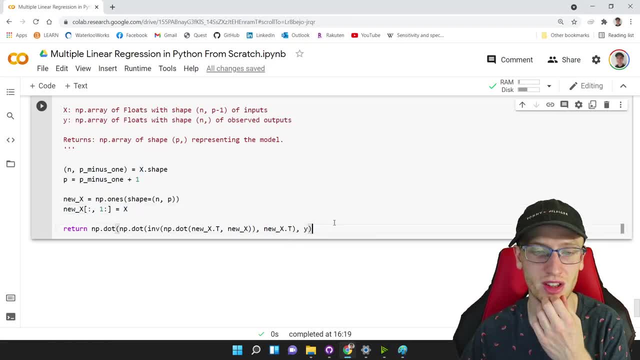 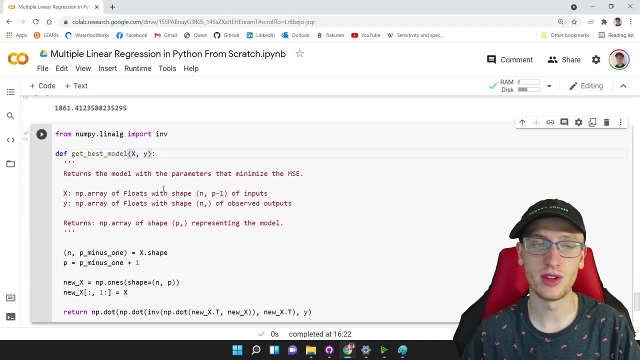 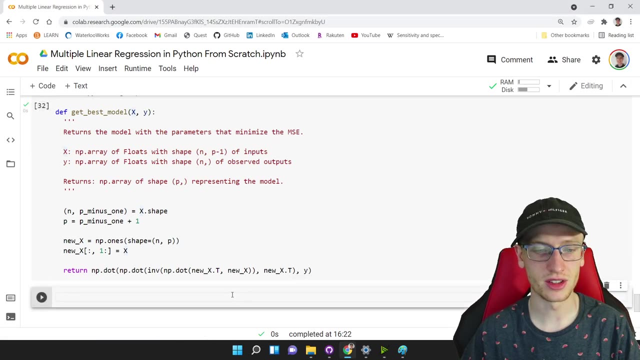 matrices with themselves. It's kind of weird. I do not want to get into that topic- linear algebra, statistics, all that stuff. So what we can do is test this thing with best model. is the get best model beating at the x? 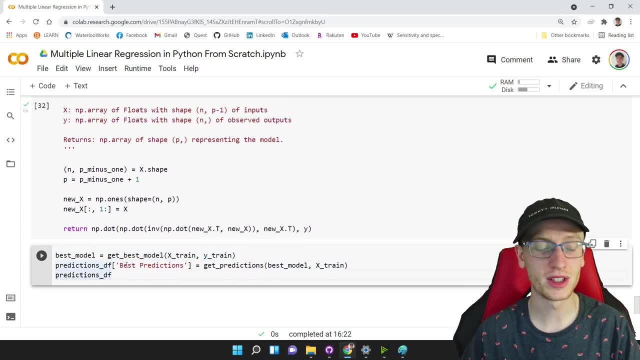 train and the y train the observed inputs and outputs. We'll add predictions df- the best predictions to be the predictions on with the best model on the training input. And then we do predictions df and we can see that our model does exactly the same thing. So we can see that our 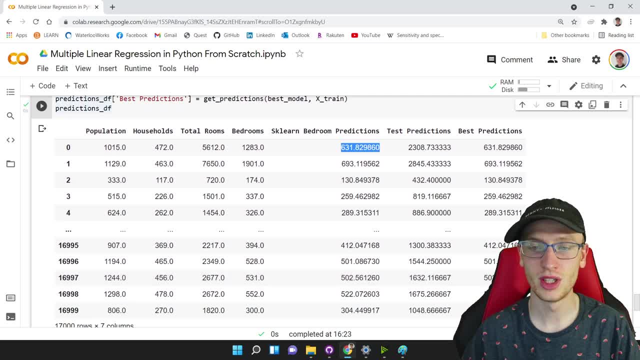 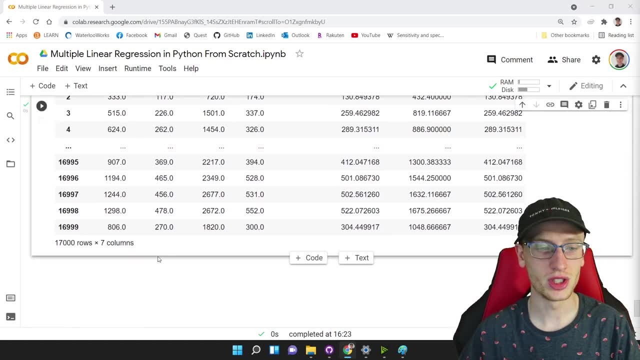 model does exactly the same thing as scikit-learn's model. it gives the exact same outputs. So it's obviously okay. All right, And if we wanted to, we could look at the error on this model, which is the mean, absolute error of the predictions df. so best prediction, so that column, right there. 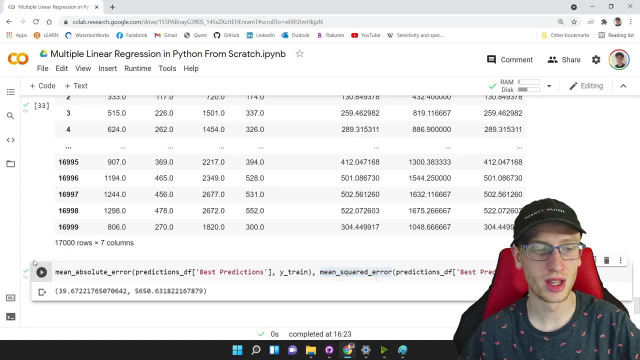 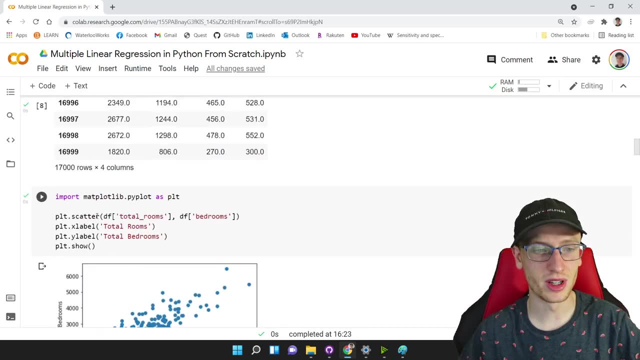 and y train and we could look at the mean squared error of it as well And we could see that it's off by 40. And 5650.. Here we see above. sorry for the headache that above we got that. where is? 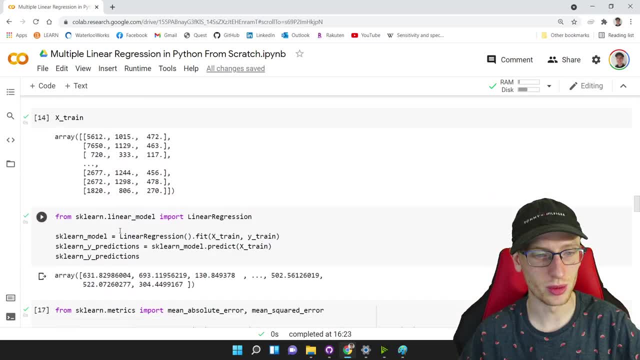 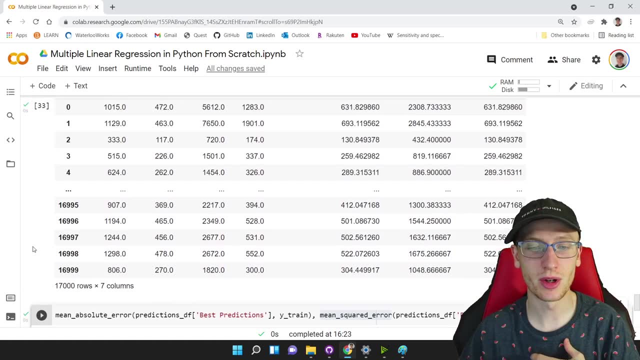 it. Did I put that right? It should be. it should be right about here up by about 40 and 5650, right there? Okay, so we made a linear model, a multiple linear regression model, And sorry for glossing. 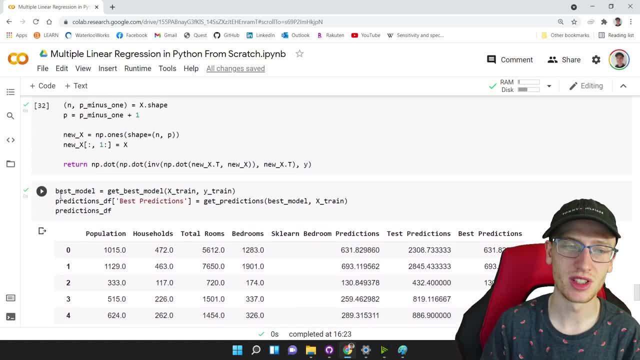 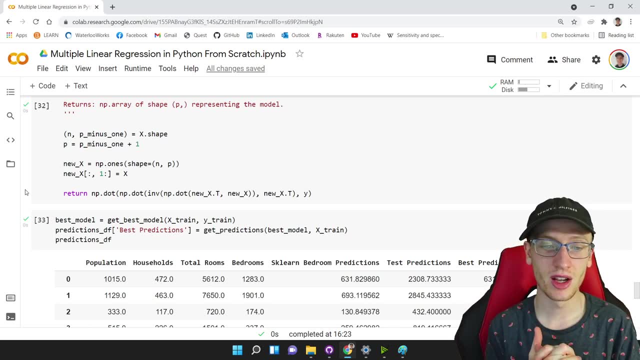 over the formula and making it looking very, very kind of skeptic. I don't like to do that, But I promise you that that was the right thing to do for this, for this video, at least in my opinion. So where to go from here? basically, we did in linear regression, it was for predicting. 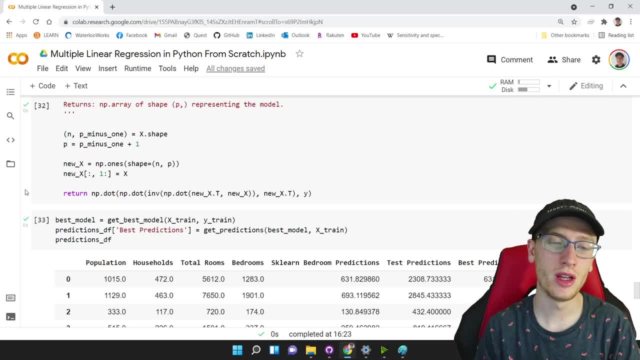 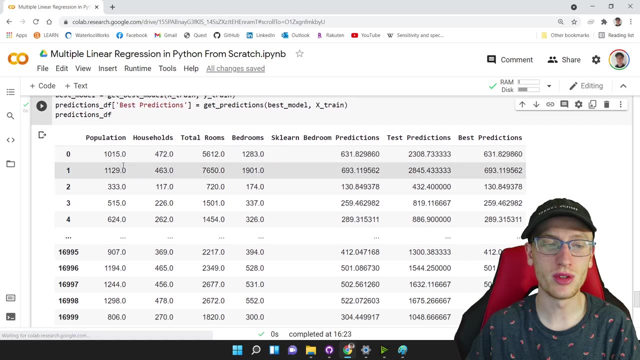 continuous values. The main point of this from a machine learning point of view, is you have a, have some inputs and you can make a linear model that predicts continuous values as well. So two things, two things to note. basically, we did only use input variables where these are. 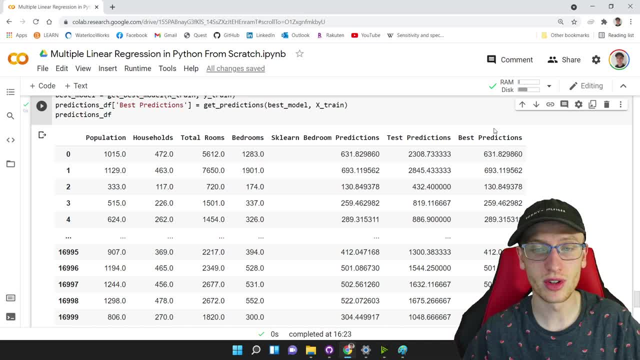 continuous variables and not the idea of binary or categorical variables. I want to do a video on that next, So that'll probably be a shorter one, But I am going to do that. how to make, how to use those as inputs as well. 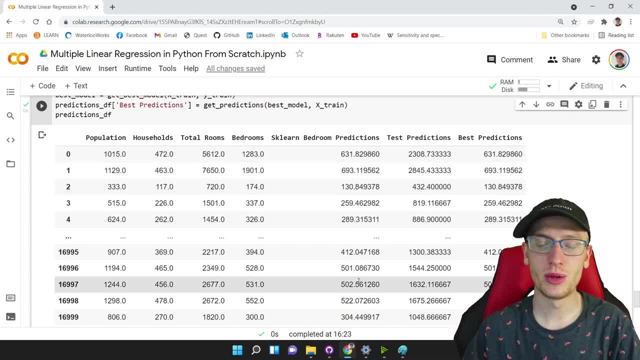 Probably the video after that is going to be. right now we're only predicting continuous values, which is just, you know, floating point values, But there's no reason why we can't do something called classification, which is trying to predict what class something is. So is this a cat or a dog? 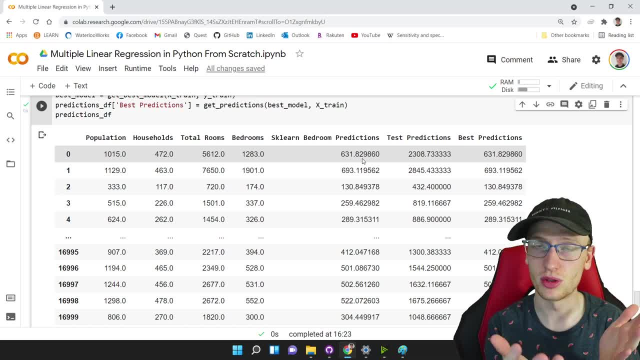 Is this fraud or not fraud? Is this? There's also multi class classification like: is this a cat, a dog, a snake, a bear, whatever? And that gets you know that actual idea of what's in a picture. 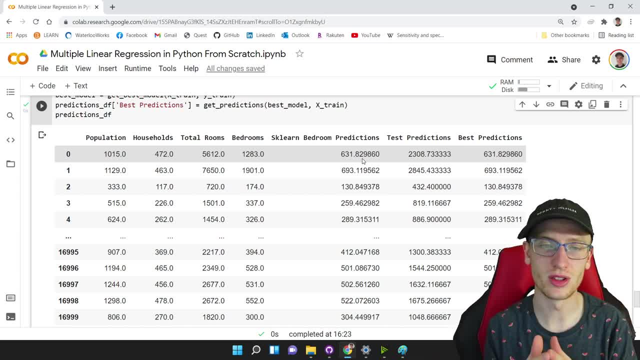 And also just we're talking about the idea of trying to predict different classes, So like class zero, class one, class two, red, blue, green, any sort of idea like that, ignoring the actual model that's used to make that. The important part is that we're changing the output So to not be a 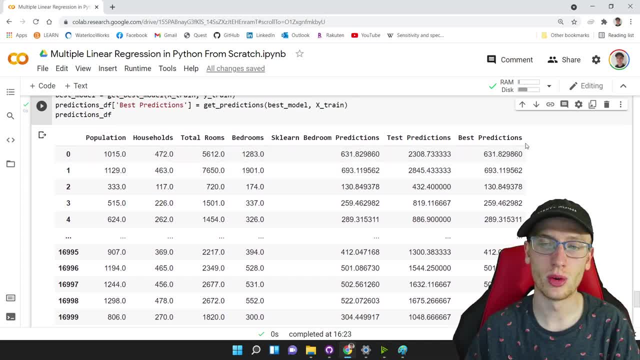 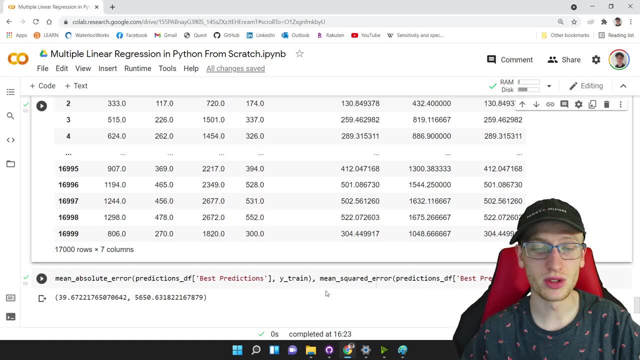 continuous value, but to be either a binary variable, so 01,, or some other class like 0123, and so on. So those are going to be two future videos. I didn't want to include how to use those two variable or how to use 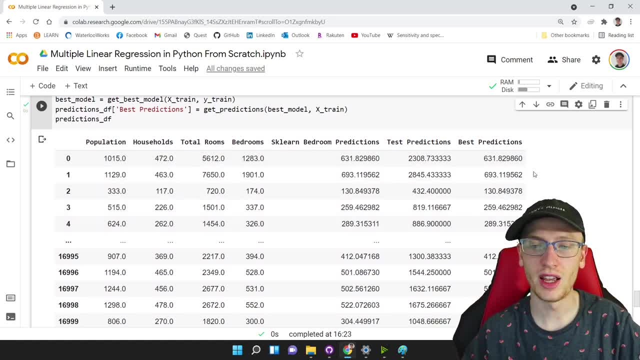 categorical variables In this video. I wanted to make a video with that own title And the one after that. we're probably going to implement logistic regression from scratch as well, And if you enjoyed the video, make sure that you drop a like and really appreciate. that helps a lot And